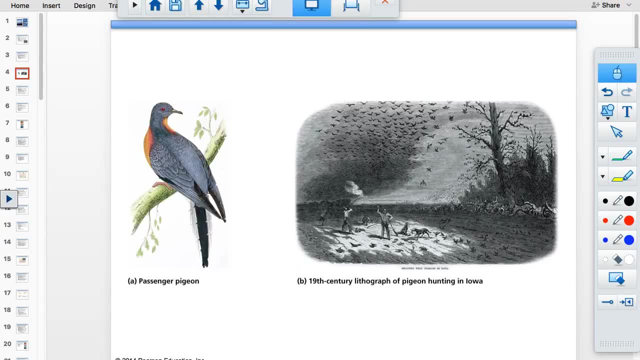 Size is the number. Nothing crazy here. Passenger pigeons: pretty cool. I had a paleontology professor in college. We talked about passenger pigeons and their behavior. I don't know if you knew this, but they were extremely populous. They would be in flocks of millions and they. 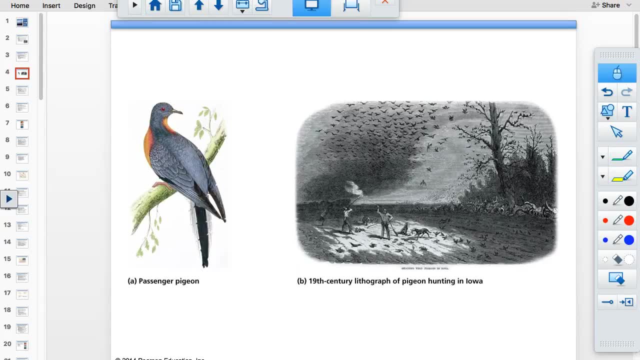 would fly over and the sky would be black for hours, And that's not a hyperbole, So it was kind of funny. The way that they reproduced was in large, orgy-like settings, And so once they started being hunted and they got down below this critical level, they could. 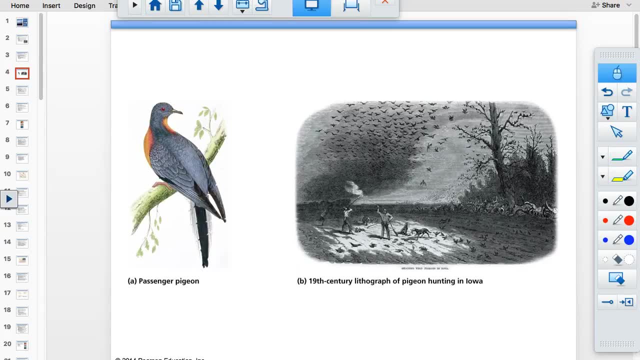 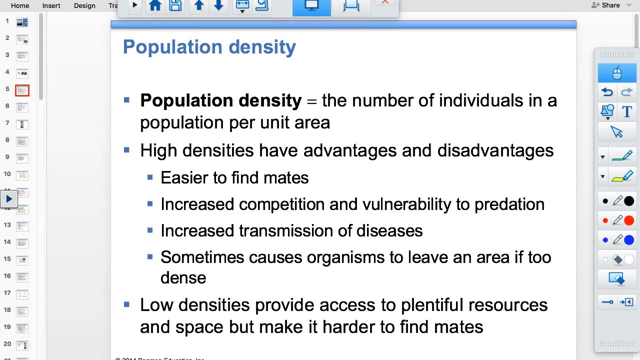 no longer engage in their traditional kind of reproductive acts and they didn't know how to handle themselves and so they all died. Isn't that fun? So I found that to be interesting, and my paleontology professor was a pretty. he was a pretty eccentric guy, so shout out. 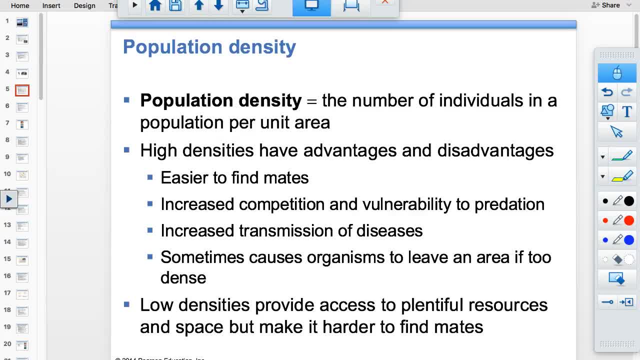 to him Population density. you'll see some questions on this on your test. That's just the number of individuals per unit of area of land, And so that's typically going to be either hectares- remember, a hectare is nothing more than 2.47 acres, Wouldn't matter. 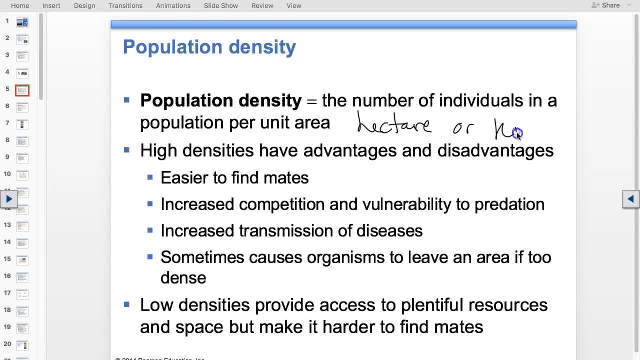 it would just be per hectare Or kilometers squared or meters squared or something. So it's just going to be individuals divided by either hectares or individuals, kilometers squared. So you would just, you know your big, your big clue there about what you need. 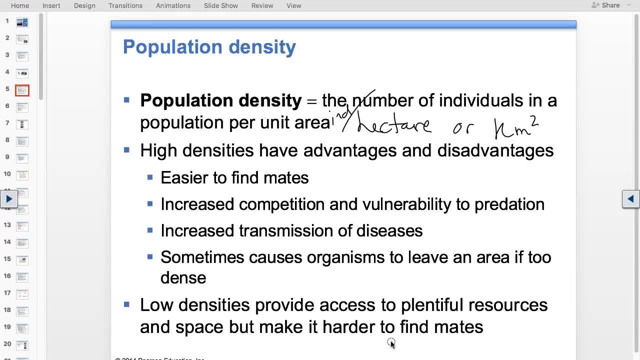 to do is: you know you're going to be able to do a lot of things And so you're going to need to see your population density and people per kilometer squared, and you know per means divide, so you just work it out. no big deal As far as the PowerPoint goes. 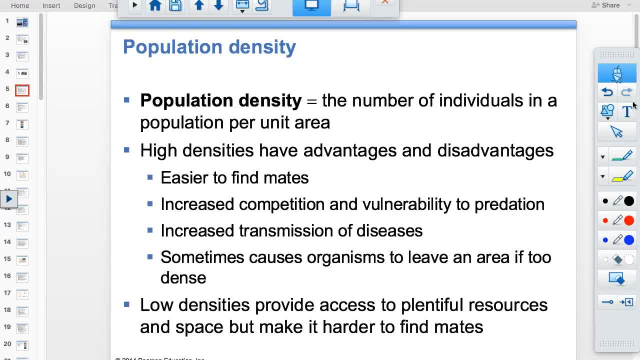 and things that you need to be ready to do on your test tomorrow. the rule of 70 is not on the PowerPoint, but you certainly had to use it in your population math right, So be ready to solve some problems with that. Remember that's just 70 divided by the growth. 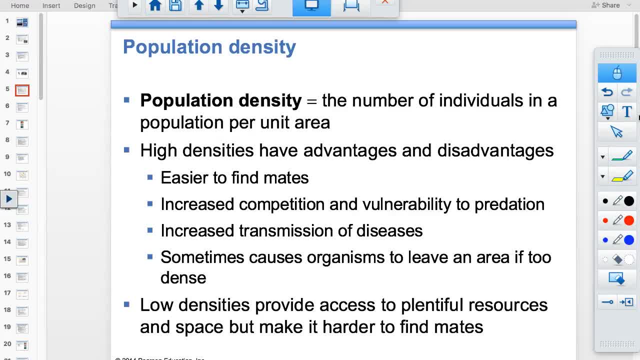 rate. Don't change it to a decimal And that's your doubling time in years, So make sure you look that up over them. Anyway, population densities- High densities- have advantages and disadvantages. If it's very dense, easy to find mates, but you're going to be more prone to competition and increased 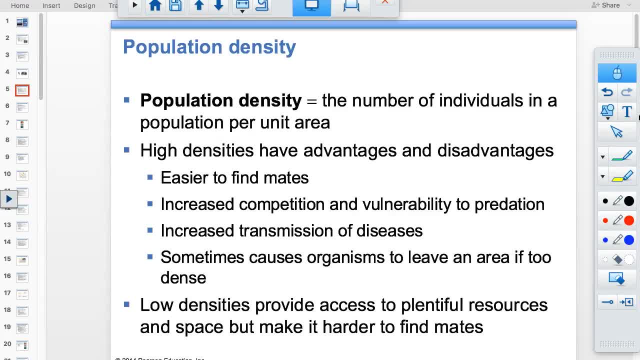 transmission of disease. That's just a good old like socialized from sixth grade, right Like the plague was from. crowded, unsanitary conditions, Low densities are good as far as finding resources, but it's hard to find mates, and so you have this positive-negative kind of situation. 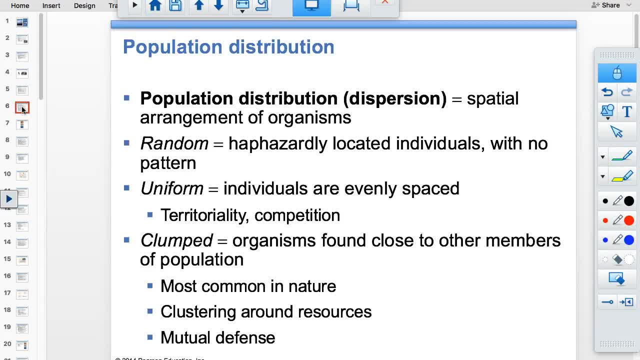 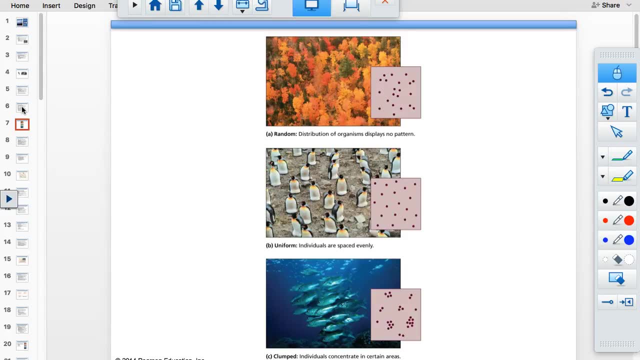 going on, where you know there's positive and negatives. So population distribution: random, uniform and clumped. This is not rocket science. Random is random, Clumped is in like schools, like fish or flocks of birds or passenger pigeons. Uniform is going to be. 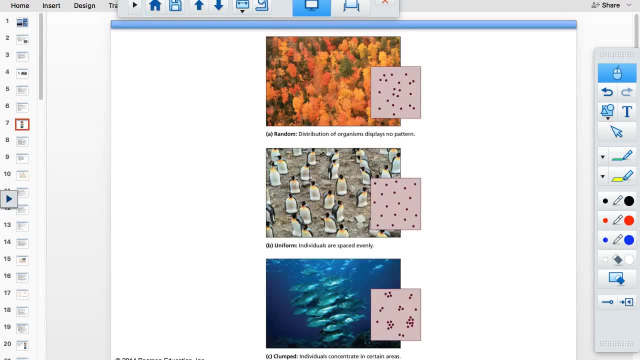 where they're equally kind of spaced here because they're having to share resources, Like trees will often do this so that they all have access to life, and there's picture The penguins are doing that, so they all have like a good-sized nesting area. So 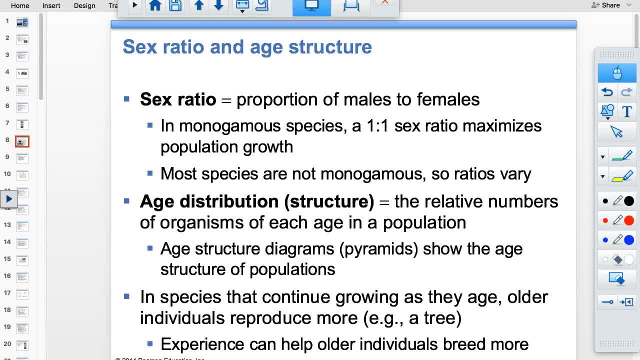 very easy. Sex ratio that's just going to be males to females, One-to-one- is going to be ideal in a monogamous species like humans. I don't need to give you like a sex ed lesson right now, but 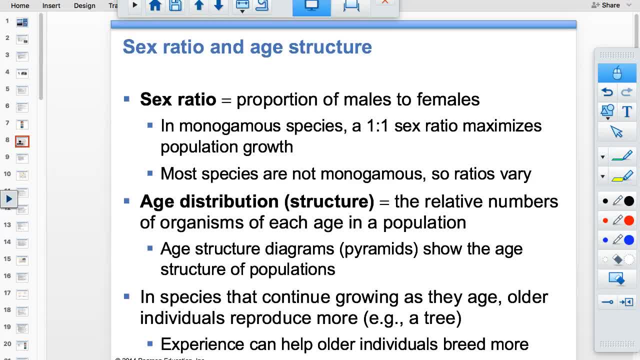 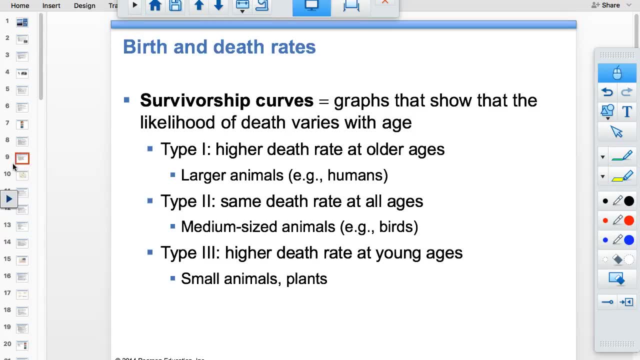 that's what we're talking about, So a distribution or a structure. those are the population pyramids that we've been looking at the last couple days and they kind of tell you the number of individuals in each cohort, Our age group. So, survivorship curves, We have 1,, 2, and 3 for your types, And so if we look at that, 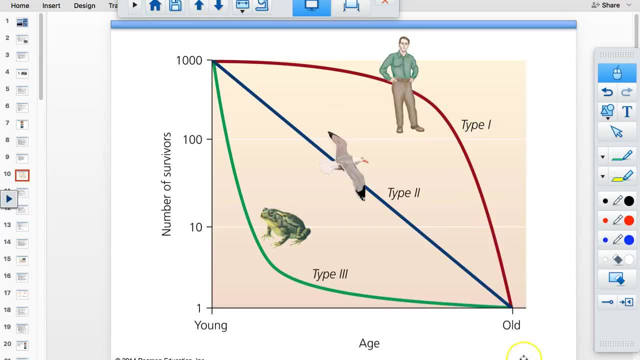 type 1 is going to be your mammals, typically larger mammals, and they're going to. if you look at the data, what this is showing you is this is number of survivors out of a thousand. So if you look up here, 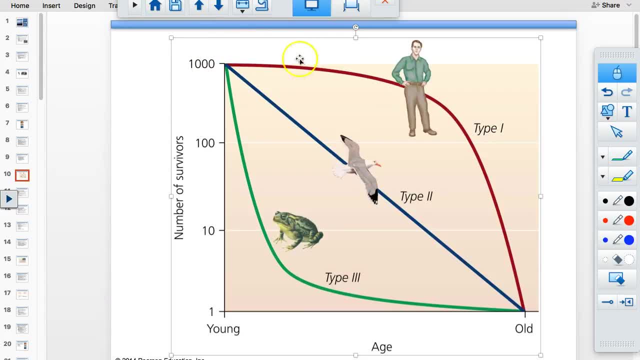 that's a pretty high number of survivors per thousand. Like, we take care of our young right And then we die when we're old in Florida. So type 2, because you have a continuous kind of constant slope there. basically birds and small mammals like 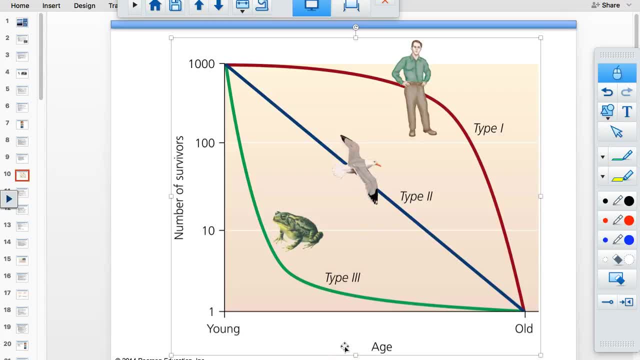 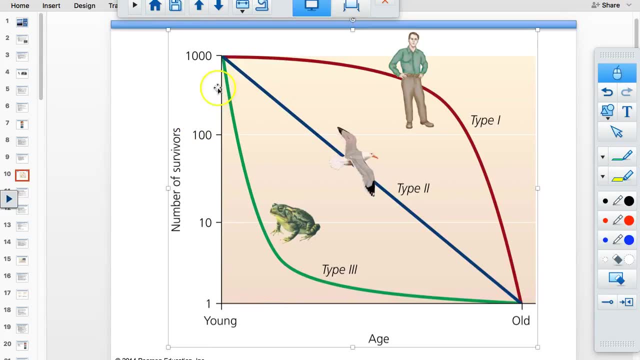 rodents. they have some parental care but they have sort of equal opportunity of death at any point. And then type 3, you can see this really precipitous whoops. precipitous drop here in survivors because they have a large number of offspring and there's little parental care. but if you're like a frog and you make it to middle. 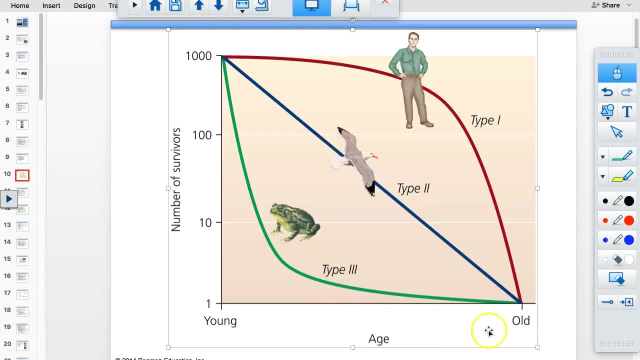 age, then you're. you know they're going to die. So that's a pretty high number of survivors out of a thousand. So it's going to be a print soon and we'll look for everyone. But so those are the three types of 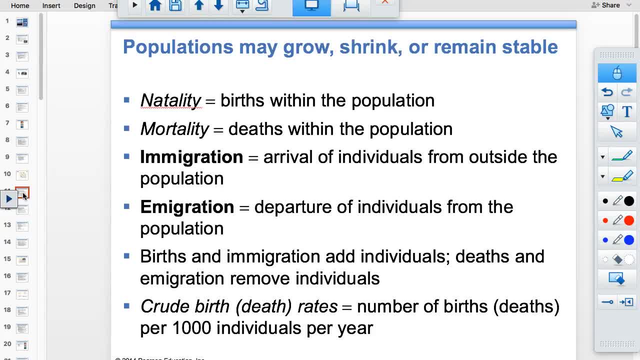 survivorship curves, Immigration with the I like coming in. So I think we already established that People coming in, people exiting. if that confuses you, that should help. As far as births, like the neonatal unit at the hospital or the nativity scene at Christmas, this little root here means birth. 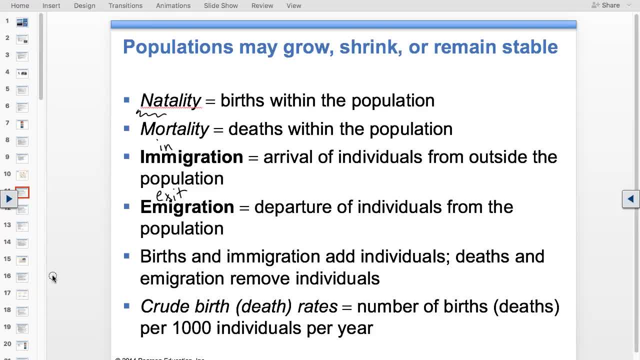 So natality is births, Mortality is deaths, And so, if we look at how to figure this stuff out, if you remember crude birth or crude death, that is per thousand, right? So if we have a crude birth rate of 6 per thousand, then our 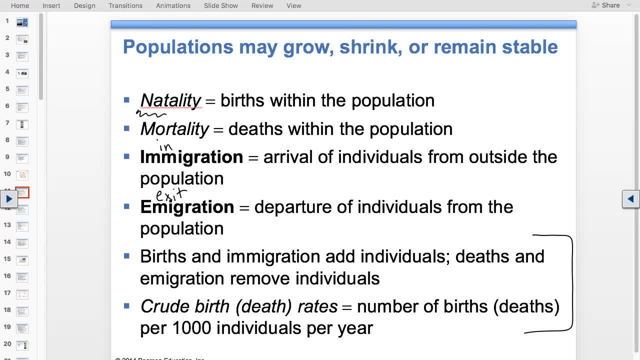 actual percentage birth rate is .6%. right, Because we're going to divide the top of the fraction by 10 and the bottom of the fraction by 10 and get 100.. If it was 6 per thousand, we want a percent. the definition of percent. 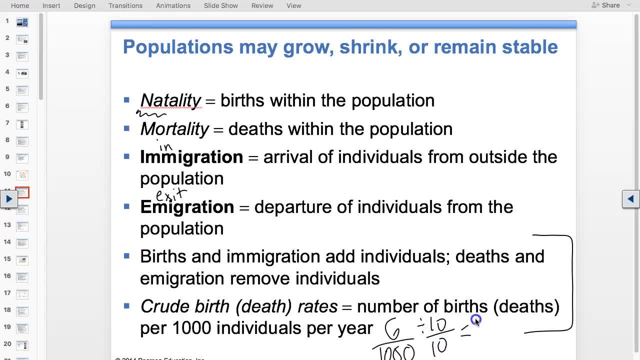 is. I guess I should do that. that makes me feel better anyway. no, no, I meant to do the birth, can I? I have that one and that's what I was going. so I have .6 over 100, which is .6%. are you going to go for it? 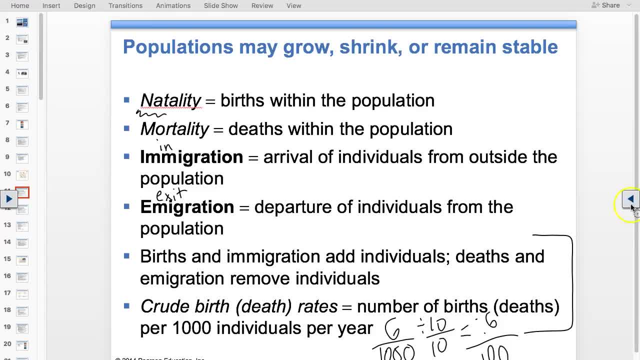 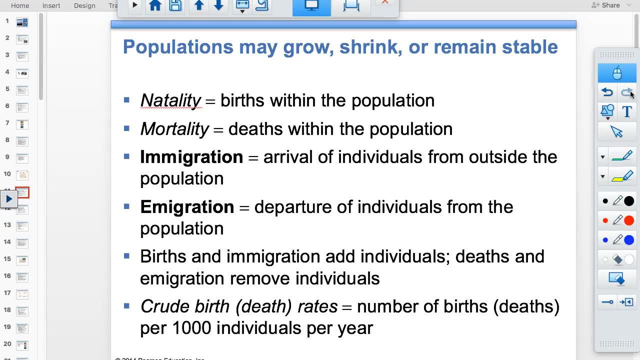 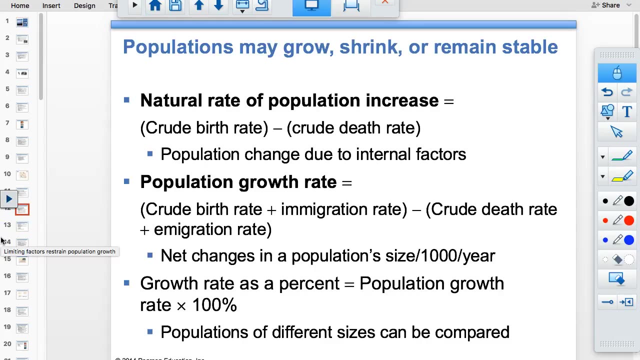 Okay, okay. so if you have accrued birth or accrued death rate, if you're given a rate, if it already has a rate, you don't need to divide by that total population. it's already a rate. we find rates by dividing by total, part divided by total times 100, or part divided by whole. so that's the biggest thing people make mistakes with. so if we're looking at natural rate of population, it's going to include your births and deaths, but it's not going to include your migration. migration meaning. 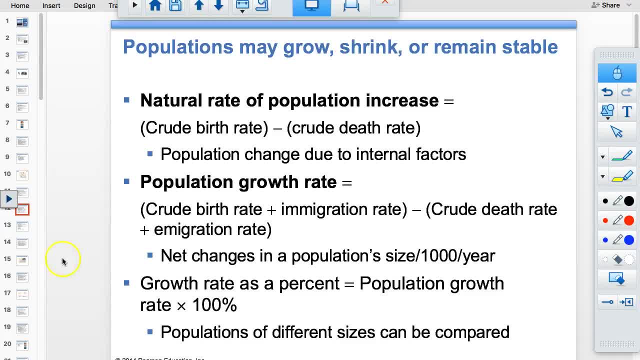 immigration: immigration with an I, immigration with an E: okay, population growth rate, accrued birth and immigration. so all people coming in minus all people going out and notice how it already says rate, it's not going to be divided by the total, it's already a rate and so that will give you in per thousand per year. if you need a percent, you would divide it by 10, because a thousand divided by 10 is 100, so there there is that information: exponential growth. exponential growth is a 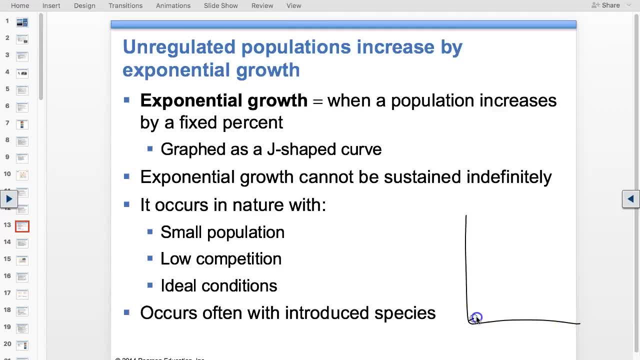 lot of space and it's going to be a J-shaped curve. so you're just going to start really low and you're just going to go like that. so a J-shaped curve is exponential, and so this really is kind of rare. it only happens when you start with a small population. it only happens for a limited time. you won't have much competition, idle conditions. so this really is. it occurs when, like a petri dish and you're growing a culture of bacteria, there's a little file that bacteria can grow exponentially because it has a lot of space, and then eventually you'll run out of agar. that's A-G-A-R, that's the sugar in the bottom of the. 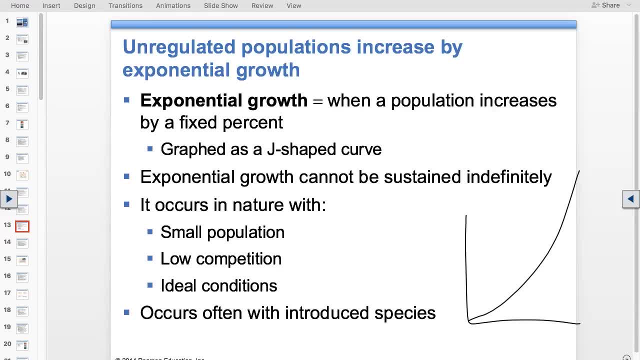 eat your dish like a kind of slime. That's sugar, That's what. that is The little substrate they use. Anyway, this will level off and so now it's going to have an adjacent curve or an edge shape curve. This is logistic growth. Exponential growth is if I don't have this curve. 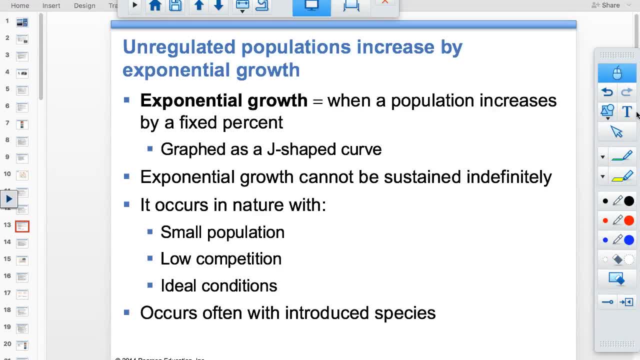 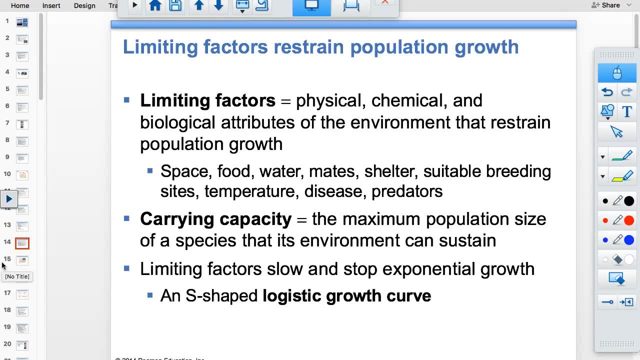 Can't go on forever, though Eventually we'll reach some kind of carrying capacity. So limited factors, The limited factors, are what's going to bring you to your carrying capacity? It can be space, food, water, mates, so it will bring site. 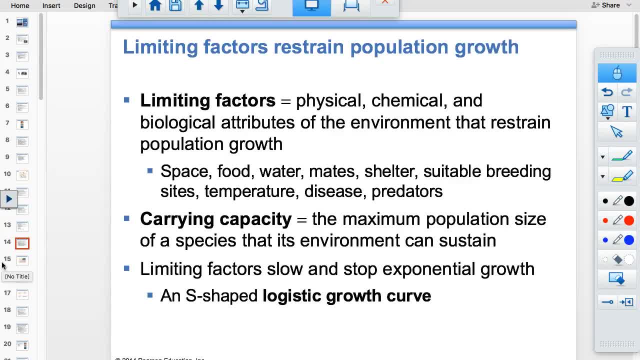 temperature, disease, pressures, and so when I level off again, that's called the carrying capacity, and it's just that maximum size that the environment can sustain. and you know, when we did the tragedy of commons lab, carrying capacity was 16 and that was the most you could have in your lake, and so you know it. 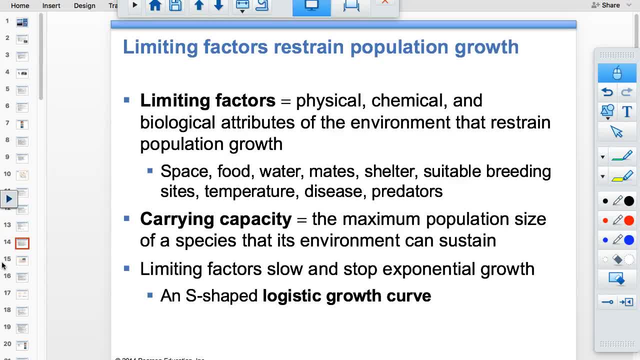 kind of keeps coming back down. That edge shaped curve is a logistic curve. How do you remember the difference between an edge shaped curve being logistic and a j shaped curve being exponential? Well, it's a logistic curve. is pretty simple. The word logistic has an S in it. The word exponential is not. 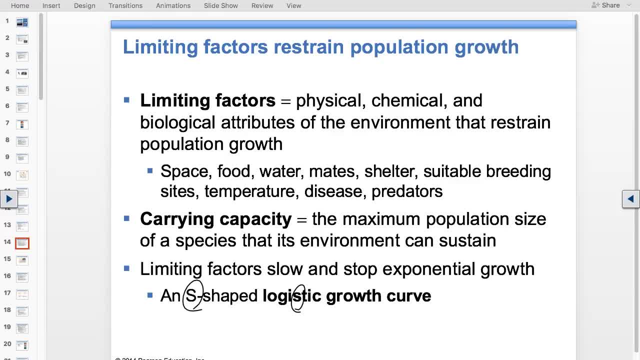 See. So S-shaped curve is logistic growth And this is what we're going to see in an actual ecosystem. They can't go on forever in a J-shape. So if we look at what that looks like and consider those limiting factors here, we see that we started with a period of that. 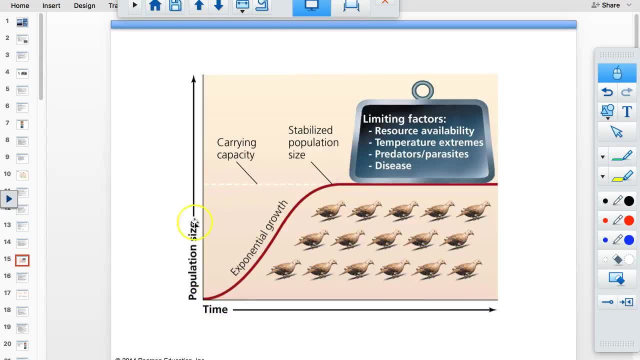 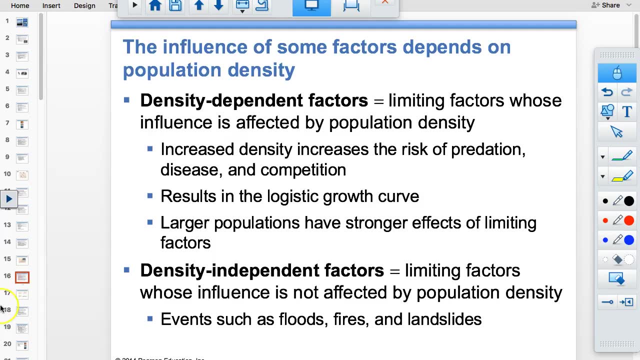 J-shaped exponential growth and then it does level off. We have an S-shaped curve. And so here's those limiting factors: resources, predators, disease, etc. Density-dependent factors. So tomorrow in your test you do need to be able to identify density. 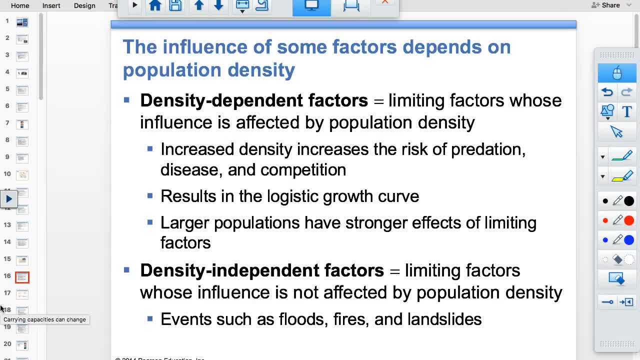 dependent and density independent. And so here's a very simple way to keep that straight: Density independent are acts of God. okay, I don't care if you have seven butterflies or 7,000 butterflies in an area. If there's a tornado come in and it tears up their ecosystem, it didn't matter how. 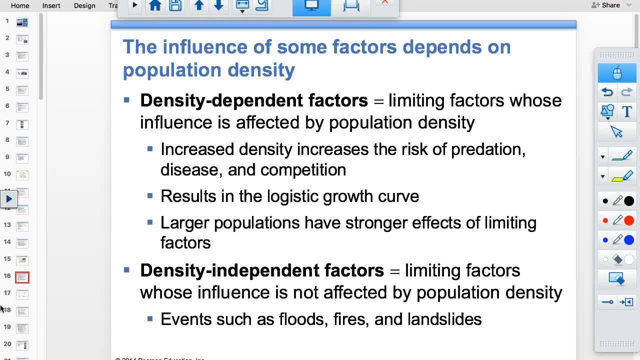 many they were there did it. It was the independent one. So if it's an act of God, it's density independent because it didn't matter about the density, It's independent of the density. understand Acts of God, density independent. If it's not an act of God, then it's. 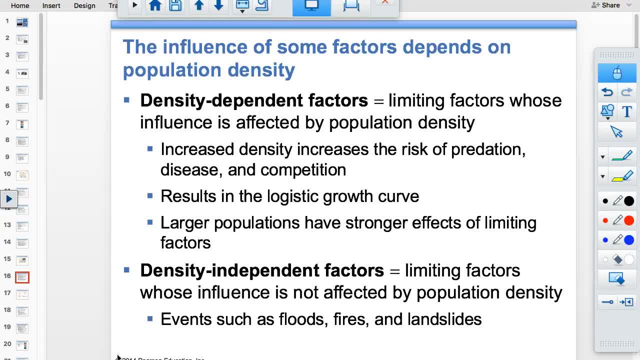 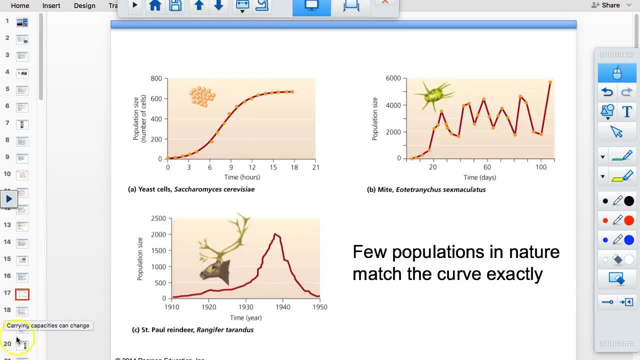 density dependent. So that would be space mates disease. Very simple, right? Can you keep that straight? All right, So here we have a nice logistic growth curve and this is some yeast cells. So if they were put into like a culture, like I said, for a while, they would grow. 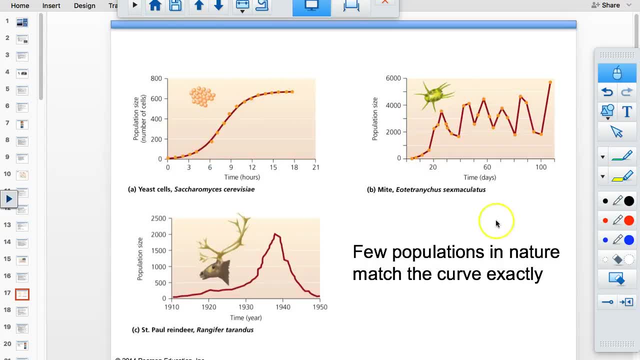 exponentially until they ran out of food or space. Not everything you know follows these curves. Mites are our selected species. They have high reproductive rates, And so if they experience a disturbance in the forest and the ecosystem, their population could come. 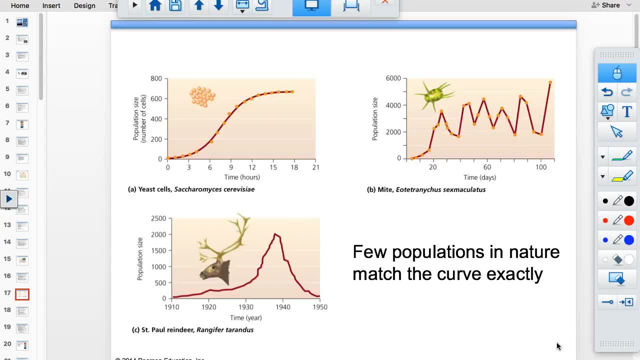 back really quickly And so pretty erratic. And then here's reindeer, and you can see that they were doing quite well. And right here is where Santa Claus became popular. But no, seriously, they probably started getting hunted, and you can see. 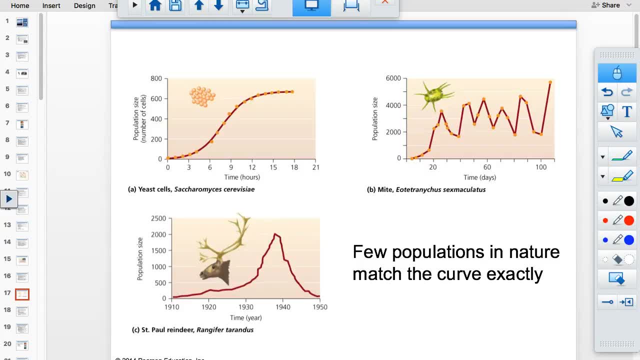 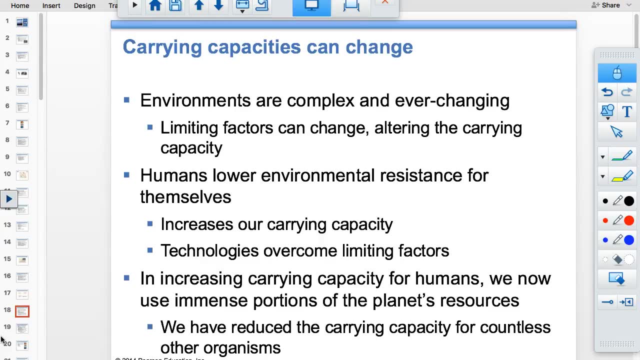 their populations. St Paul, reindeer, I just it's a nice name for an animal, Sorry, they all did now. So our myths are changing and technologies For humans. we're really good at increasing our carrying capacity because we have technology, So of course we're going to talk about that later. 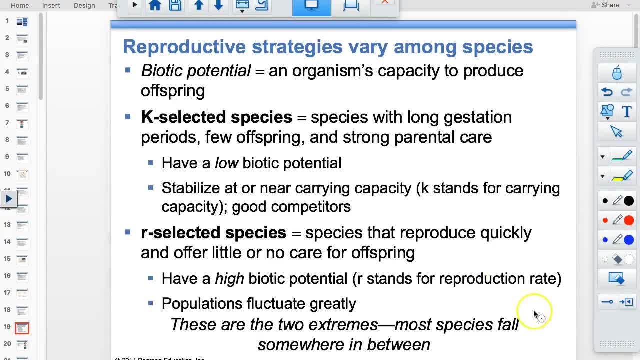 So those K-selected and R-selected, Just to kind of reiterate what we've already talked about. K-selected are like kangaroos, right, They have a few young ones. They have a few young and they care for them in their little pouches. K-selected species don't have to be. 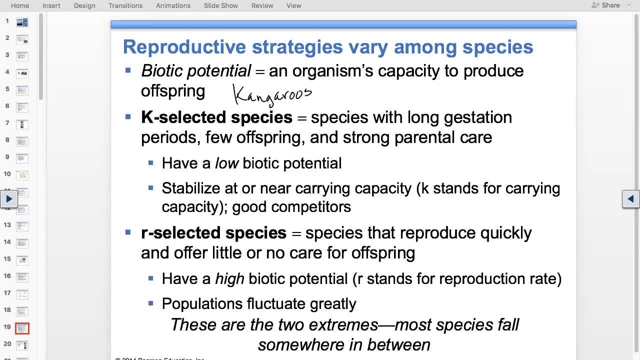 kangaroos. I'm just really talking about any organism that has a few offspring at a time. Cares for them Takes a long time to mature. So long maturation That means that you know, can't reproduce it for three days. It would take, you know, 30 years. 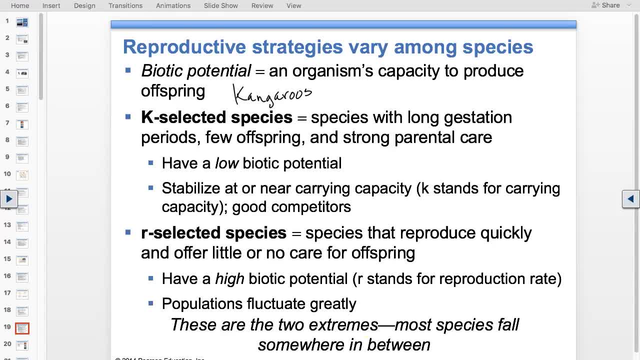 Not thirty years, but you know 13.. Our selected species are like roaches: They have a lot of young at one time, but a lot at a later time. The older ones are a little younger, A little older. So they that's. you know. they have more. 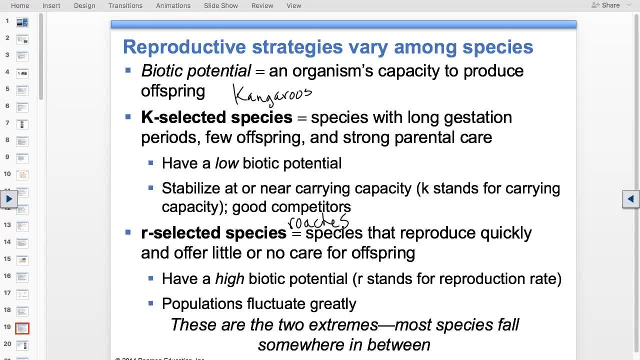 little parental care. So why did we have the K and the R? What is that even about K? I don't know if you know this, but like German doesn't use the letter C. Well, now you learned something today, didn't you? So K in German, like the KT, extinction the word. 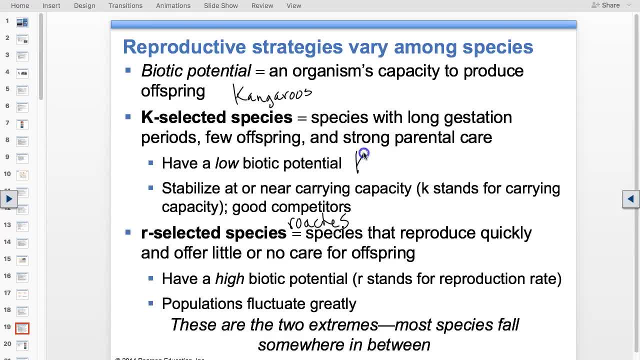 Cretaceous starts with a C, but in German it starts with a K. Anyway, K stands for carrying capacity. So K selected species are not named K for K roots. they're named for K because their population is going to level off at carrying capacity and remain pretty. 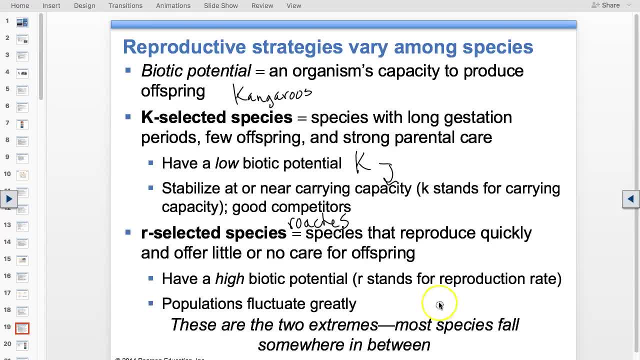 stable. Our selected species have a high reproductive rate, okay, and so that's why they're named R-selected species. So if you see the letter K or the letter R, you have to understand what that means, not just like words, books, okay. So, and that's. 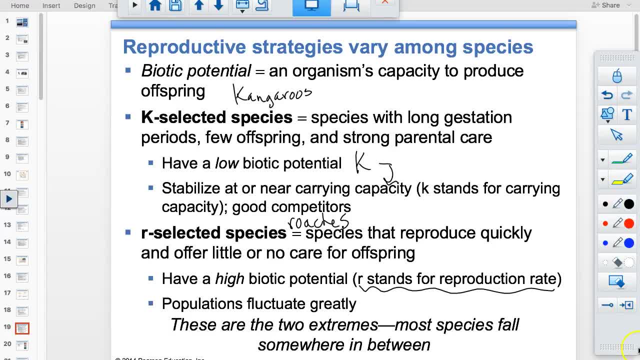 extremes. They're not. not everything falls into these two categories, but a lot of things do So. biotic potential: if you see that that means you have a high life potential, You can have a lot of babies. That's really if I wanted to make. 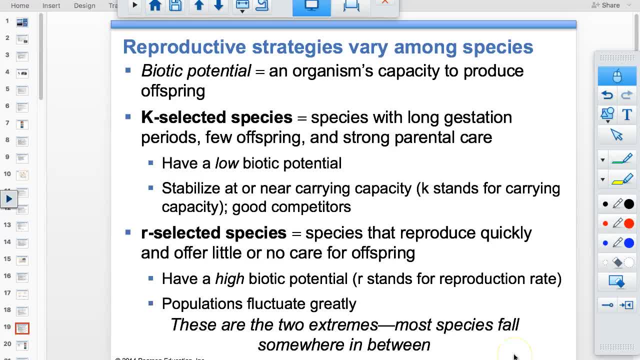 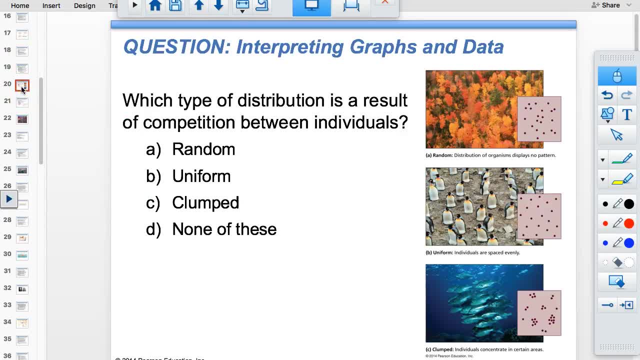 it simple for you. that's what that means: How we feeling: Heavy times, All right, um, let me scooch this on down. So let's answer these little quick questions at the end here. Which type of distribution is a result of competition between? 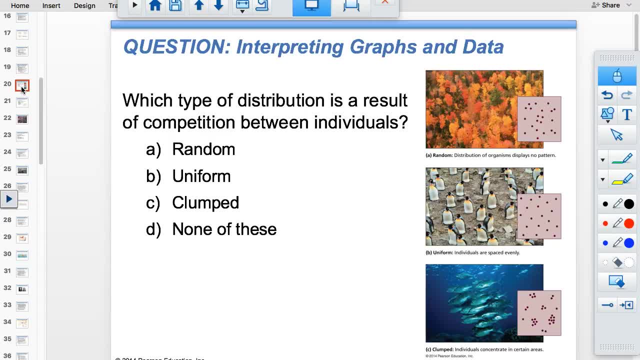 individuals. What do you have, Coby? Yeah, and so they're gonna space out um space, become evenly spaced, that share resources, um. so what does this graph show? circles on the line? uh, just kidding Ashley, what you? 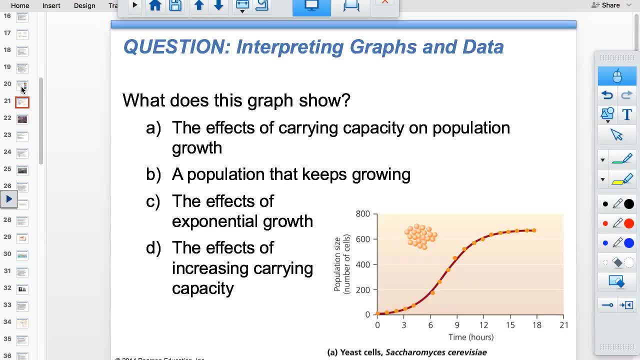 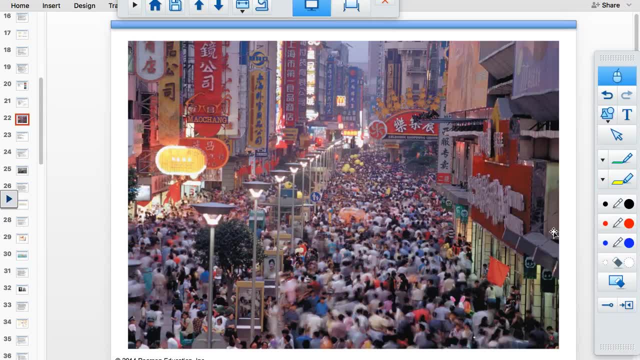 got, Yeah, so the effects of care and capacity on growth. and so you can see, here's the care and capacity and the growth does slow down. and so now I have China. yay, So after January 1 2016, the one child policy in China is now a two-child. 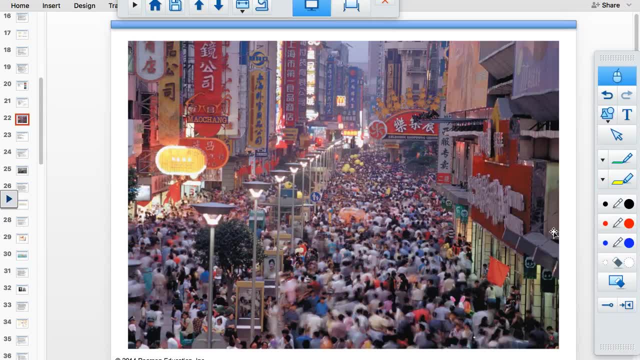 policy, and so the AP exam really likes to ask questions that are from last year's current events. so I really expect to see some water pollution problems in Michigan on there, and I really expect to see China and the one-shot policy. they haven't asked a population question in like eight or nine years, like it's. 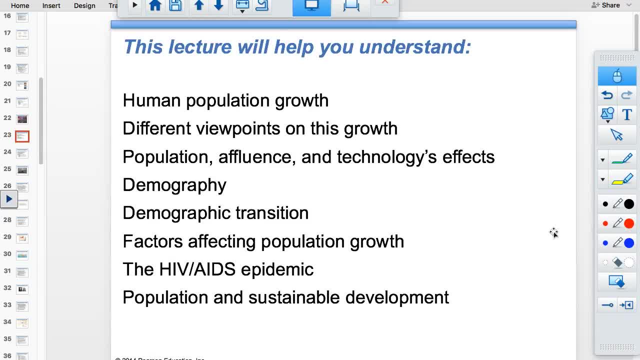 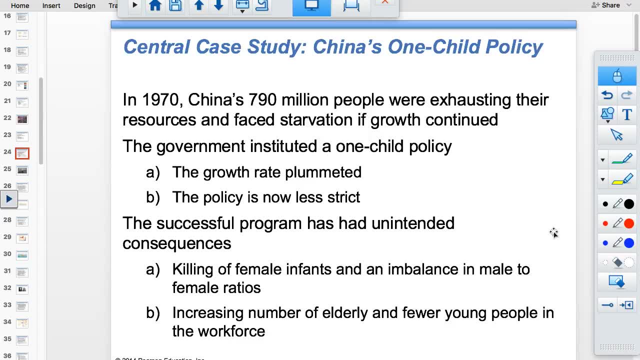 overdue. so a human population is kind of where we're going with this, because we just covered like biology basics. so in 1970 time was just coming out of a famine sort of stricken kind of situation where they had a lot of people starve to death. it was awful, and so before we sit here and like say oh it's. 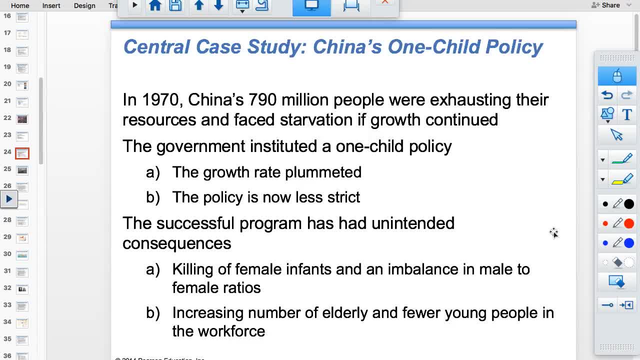 terrible that they make you have an abortion or they aborted their female babies or you know they're kidnapping people. the countryside for wives like that's. that makes us sad. but you have to understand that they took these measures to instate the one-shot policy because their country was overcrowded and you 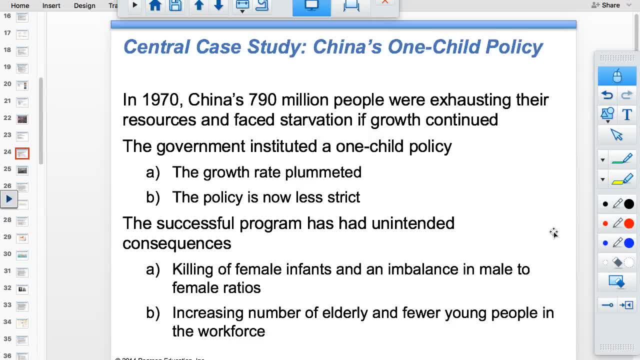 know those people were starving to death, right. so they took measures and they were pretty drastic and quick and they were- maybe were they inhumane, but so it started to death. so it's really important when we look at these issues that you kind of ditch your cultural. 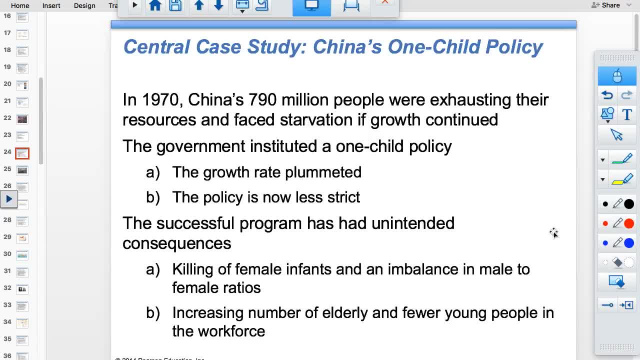 preferences and think about it from maybe their perspective. crazy talk, right? so, anyway, one-shot policy. the growth rate plummeted and now the policy is less strict. and now so it's even less strict. now you have two children, right? so because of the cultural preference for male children, there was a selective 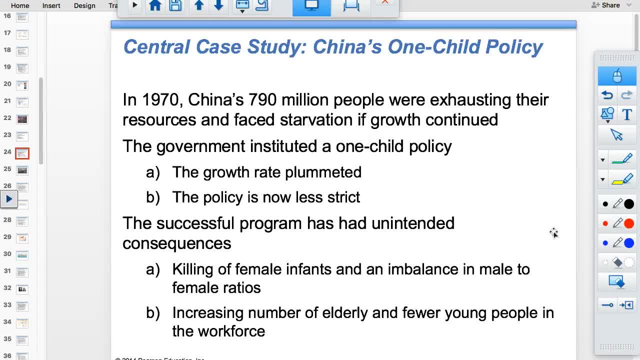 abortion of female infants, and then there was some some forced abortion of female infants, and then there was some forced abortion and then there was some forced sterilizations. then then I did also tell you that you know, the second child, when they had the one-shot policy, did not receive all the same rights with the 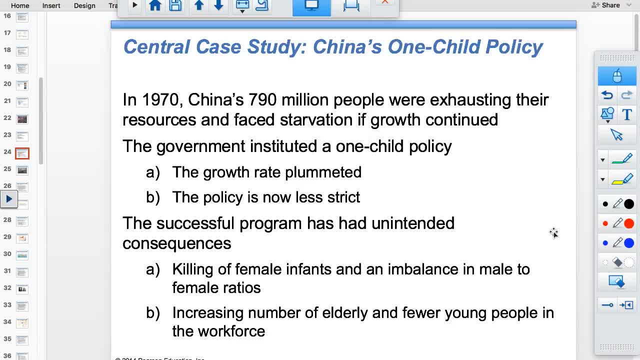 free education and care. so there was fines involved. in some, depending on the area you're in, there were some sort of manipulative things done to to force abortion or forced sterilization. so anyway, the issue now and the reason they have moved to the two child from one child is because when you have a society, have 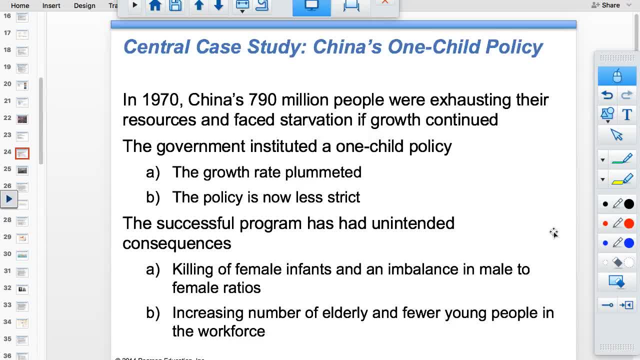 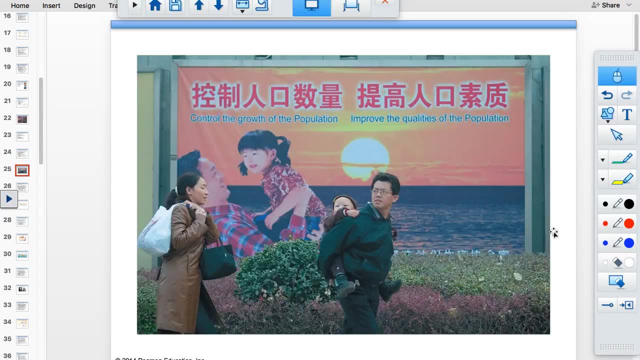 these elderly people, they're going to need social services and they're going to need health care, and so it is the working-class people, those reproductive age people, that are paying taxes, and so increasing the workforce was, you know, kind of needed. so then, a lot of propaganda in China, with you know hey. 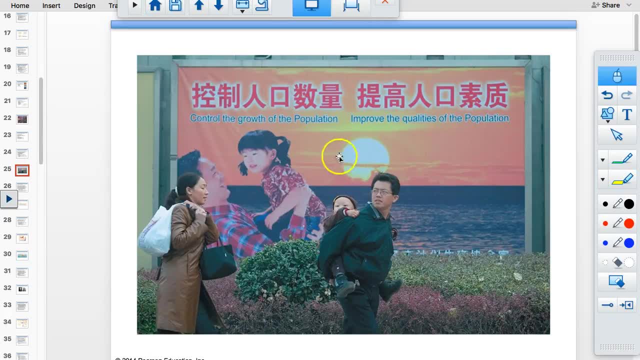 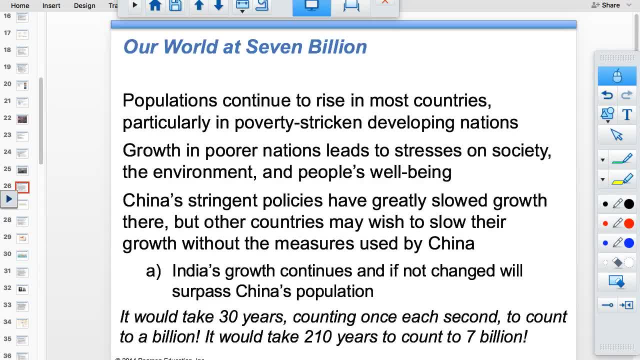 the main issue, though, as we continue to see the world's population grow- it will peak at about 10 billion in about 2050- is that 99% of the next billion people, and that's- I'm not making this statistic up- 99% of the next billion people in the 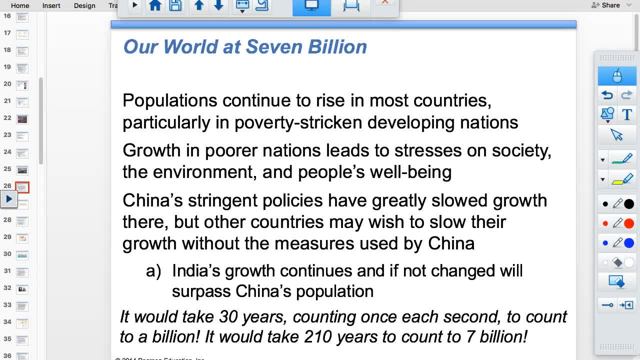 world will actually be added to the developing countries that cannot support them, and so poorer nations tend to have, tend to have the highest growth rates, and so I mean we talked about some of those factors, but we're, you know, going to get that India's growth rate is. 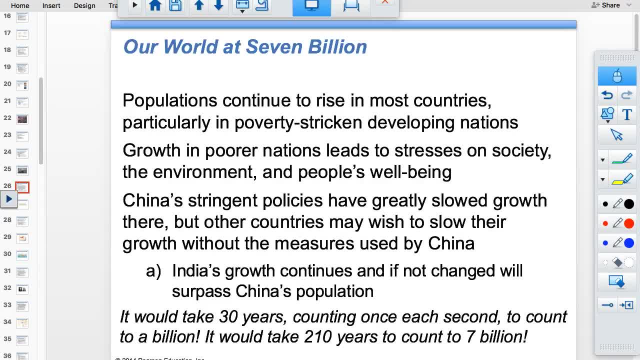 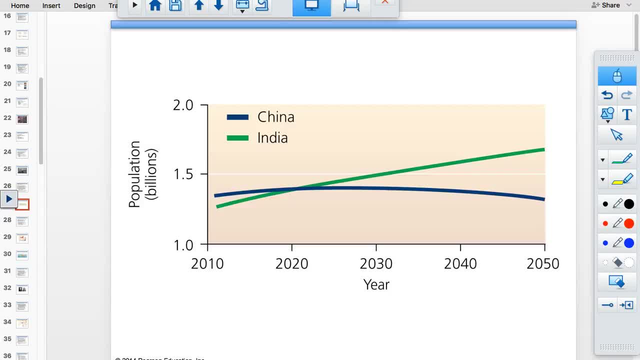 continuing and it's gonna surpass China's population. in the next decade. they'll actually have more people than China, so if that's a race, they're gonna win. okay, so here's a nice picture. so, like I said, in the next decade, India will surpass China and continue to grow where China's population is pretty. 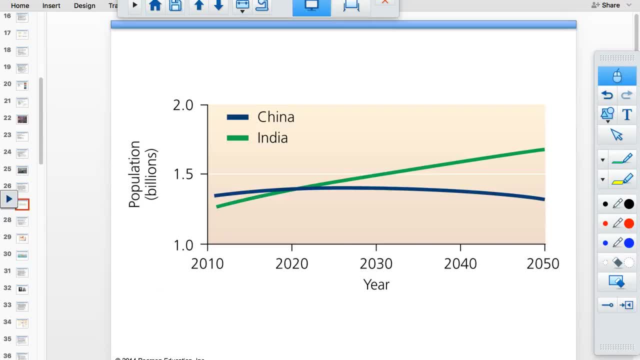 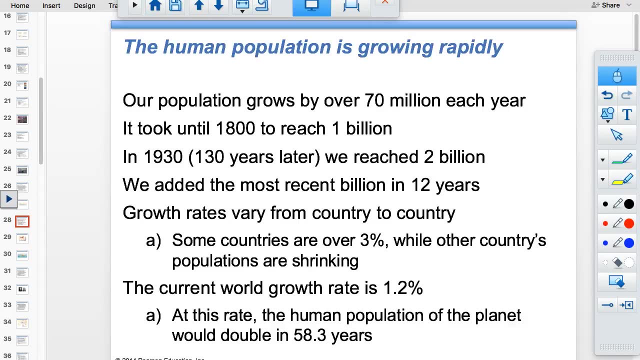 stable now and it will start to shrink. so kind of scary population grows about 70 million each year, and so when this PowerPoint was made, and I think when I made your test, the population was 7 billion at 7.4 billion now. yeah, so that's fun and so we've. 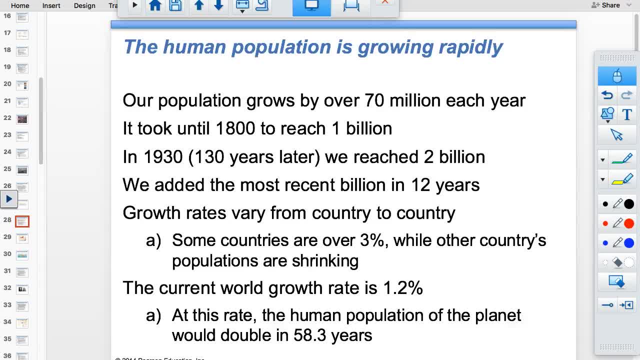 added the most recent billion people in the last 12 years. just do that math. so humans are hominids, humans and human ancestors been around for like two million years and it took us 2 billion years up until 1800 to get to a billion, and then we've gone six and a half billion more people since 1800. I'll talk about the six and a half billion years since 1800. 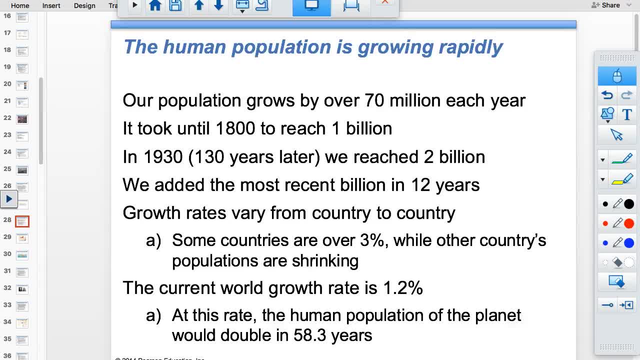 so it's very much a we're at a logistic- oh, excuse me, we're still exponential. we haven't hit our carrying capacity, but it will happen in your lifetime, right as you're in the prime of your life. so I wish you well with a retirement and I 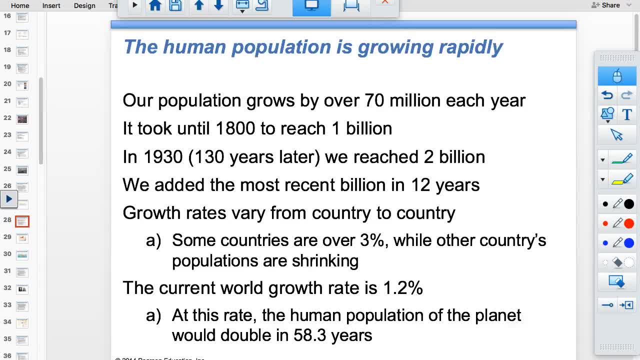 wish myself well too. so, anyway, if the growth rate is 1.2 percent- and so check this out- if it didn't tell us how often the population would double, you can figure that out right, because 70 divided by 1.2 is equal to 58.3, so you. 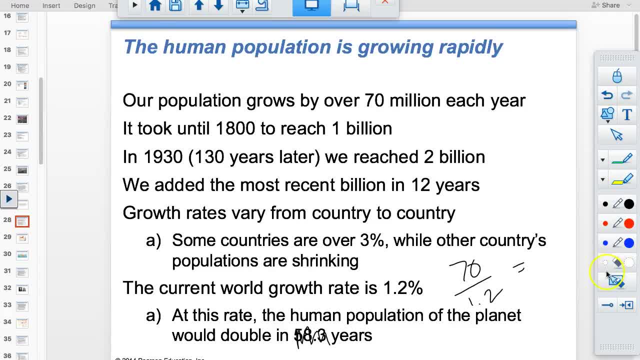 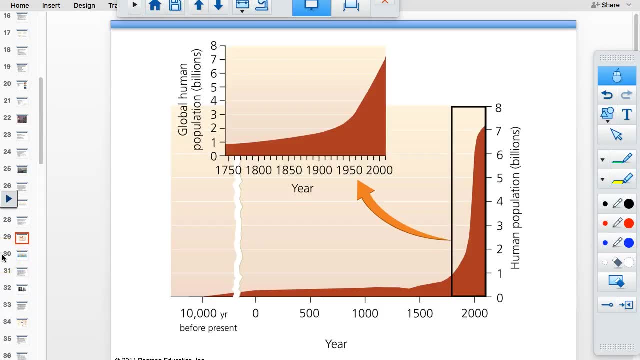 feel okay about that. and if also it had said that the population doubles every 58.3 years, you could also solve for X, so be prepared to do that. just little reminders. so if we look at that really beautiful J-shaped curve and so we could go, it took us until 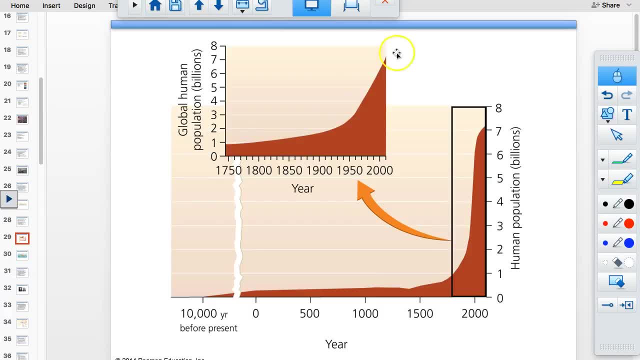 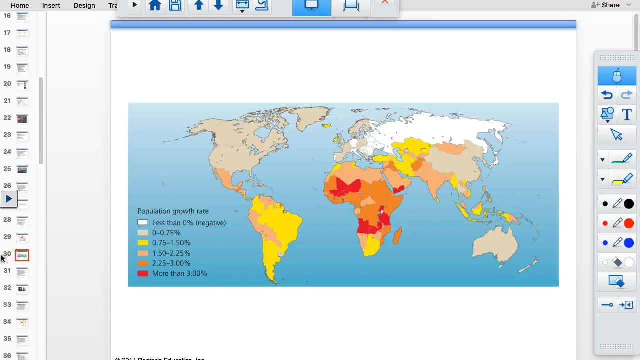 1800 to get to a billion. so if we zoom in, you can see that we're very much still on a fast rate here. and so where is this growth happening? it's mostly happening in developing countries, particularly those in Africa, Asia and South America, Africa being the fastest growth rates because they're the poorest. 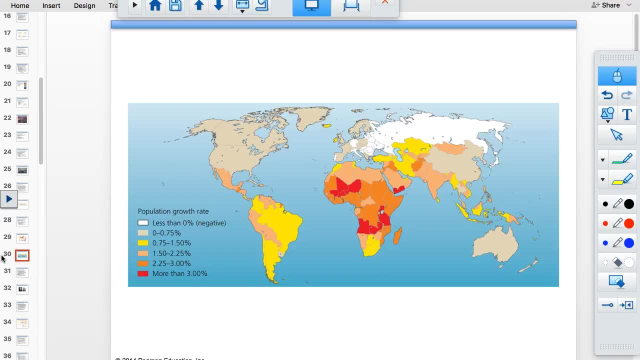 countries and so, please, it's kind of counterintuitive that the poorest countries have had the highest growth rates but poverty and patriarchal society have not been the fastest growth rates in the world. so it's kind of a they really go hand-in-hand, because you've taken half of your population and 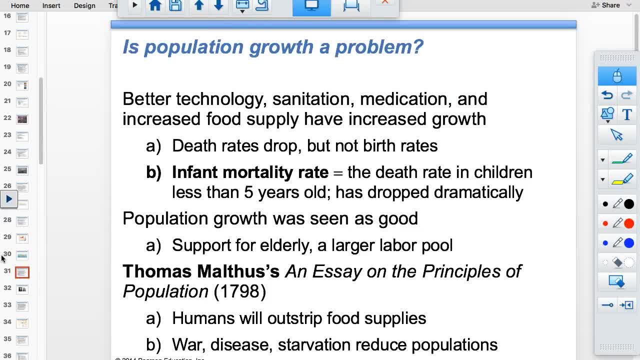 you've restricted them from the economy. so what's happened is, with our increased population growth is that we, as a global society, we don't like to die, okay, and so people are really into like not dying. so we're real, yeah, and so we're we're big. 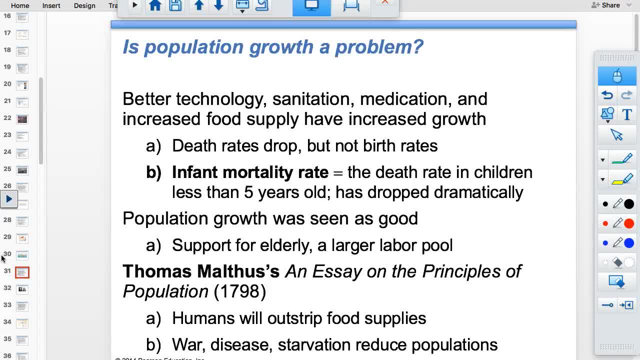 fans of taking technology and growing more food and figuring out: hey, it's probably good time then wash our hands and do immunizations, those kind of things that keep people- immunizations are actually a thing- but that they actually work. anybody got polio? no, okay, so those things are dropping the death rate. 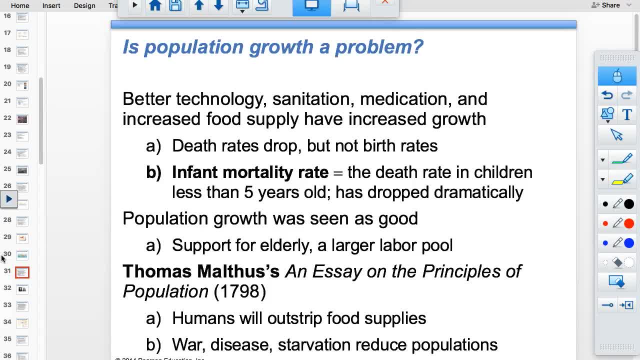 great. so it turns out that people are cool with, like, washing their hands and having dinner before. they're cool with, like, when they go into school and having birth control, and so we're still at the point as a world overall where you know, like 70-80% missing kids are out there, like 70-80% left out. and plus almost 300,000 chocolates who lose their lives. that took it wasиль'sний. see the harm is it did that a lot ofachtenheit DR disease does my horos Day. I'm basically being câmera in those situation. that's something that I started doing, but point out that it's easier with 80%, which brings over it easily. so I just for your analysis: in life I don't want to do calories free food diet. 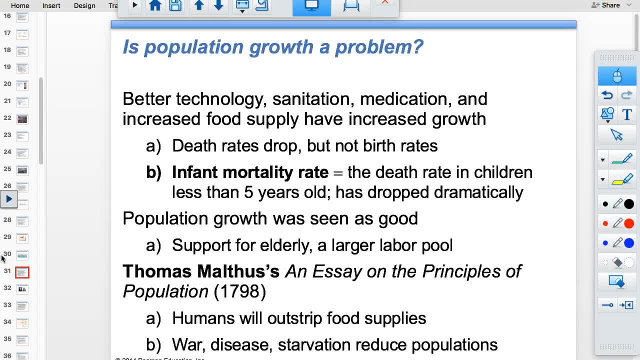 The death rates have dropped but the birth rates are still high because of opportunities available to women. So population growth traditionally was seen as good because you needed support for the elderly. There was not Social Security, There was not retirement plans, So you needed people to take care of you in your old age. 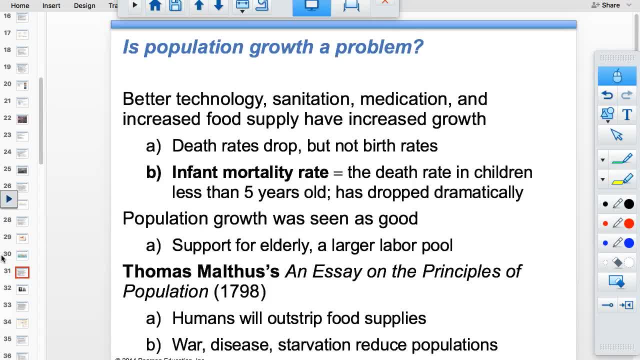 And you needed a large labor pool, because a lot of society up until the last 200, 300 years was subsistence-based, where you farmed your own land and fed your family, And so you needed kids to work on the farm. So it wasn't until right at 1800, where we hit a billion people. 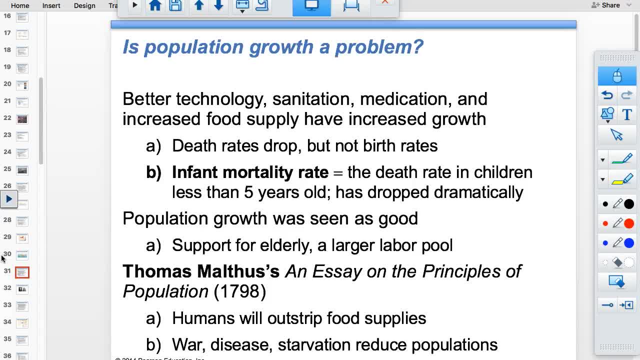 that Thomas Malthus kind of came out and said: hey guys, all these people, it's not so good because we're going to outstrip food supplies and warn disease and starvation. It's going to reduce populations. I have a song about him. 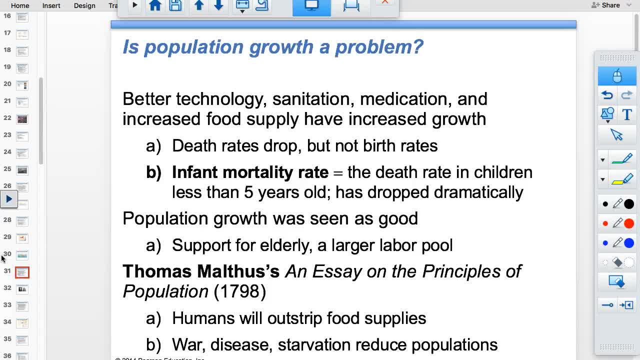 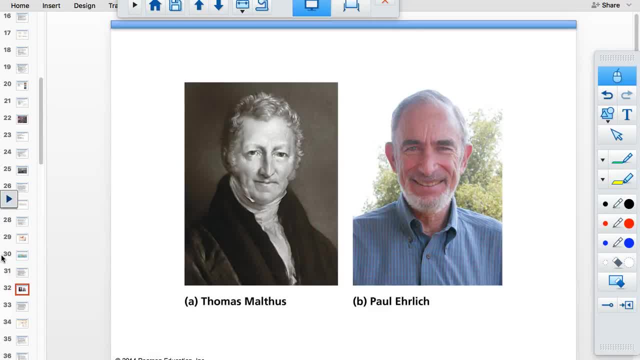 I wrote one here. Okay, Malthus was an economist man who said: what really need is to stop having so many kids or we'll all get diseases. Okay, So here's. Here's Thomas Malthus and here's Paul Ehrlich. 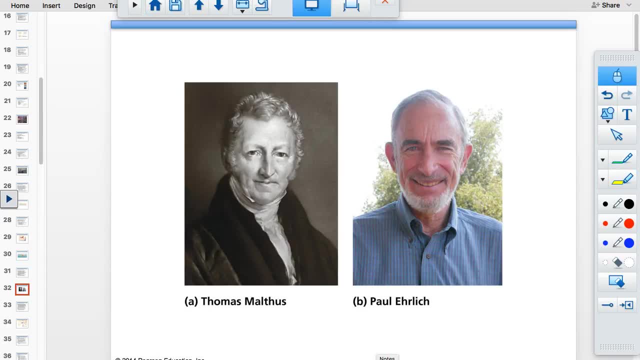 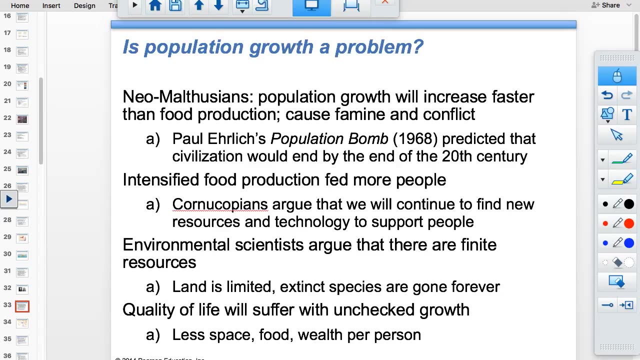 He wrote The Population Bomb in like 1968. And he was called a Neo-Malthusian. Neo means new And Malthusian was obviously referring to him. That's on this next slide. Sorry, I ruined the fun for you. 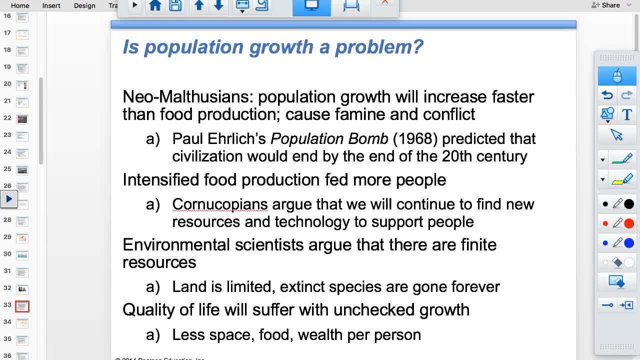 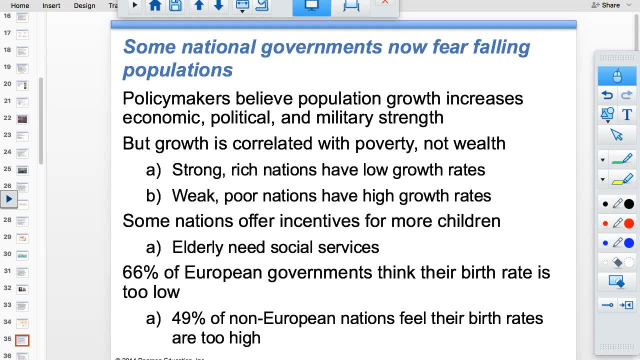 Anyway, as we have more people, we kind of obviously will have problems with less space and food and wealth per person. So here's a graph I'm not going to talk about. As far as International kind of opinions on birth rate, most European countries- about two thirds of them- feel like their birth rate is too low and about half of countries not in Europe feel like their birth rate is too high. 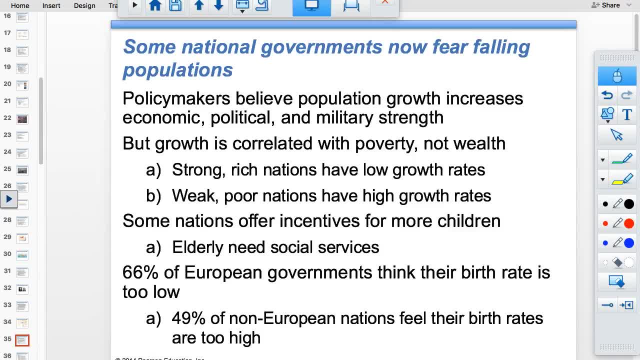 And then again for like the third time in the last five minutes. growth is correlated with poverty, not wealth. Okay, Strong, rich nations have low growth rates because they have better education systems And it really takes a lot of money to raise children in an affluent society. 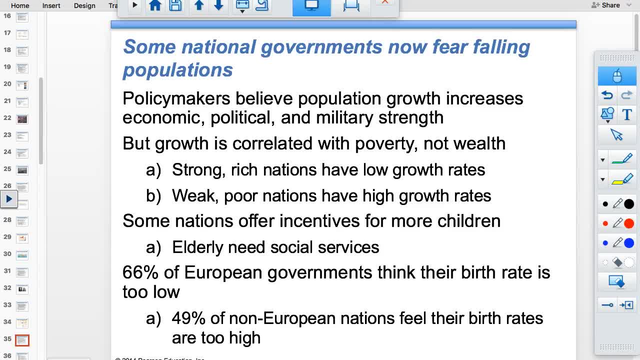 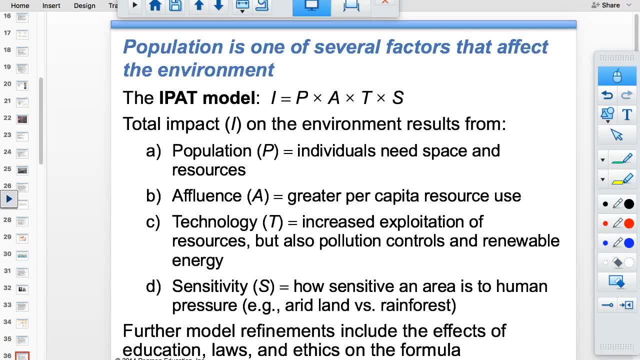 You've got to send them to school. Yeah, They want to play soccer, want to play the piano and they want to, like you know, eat pizza rolls, And so that's a lot of money. Wait, pizza rolls in my. it bought me yesterday. 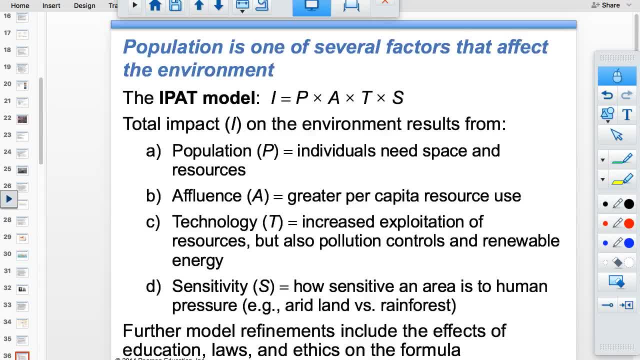 I was like: no IPAT. So remember you can pat your eyeball, Actually close your eye first, But IPAT. So the IPAT model is environmental impact is equal to population, So just one part of this is actually the number of people we have. 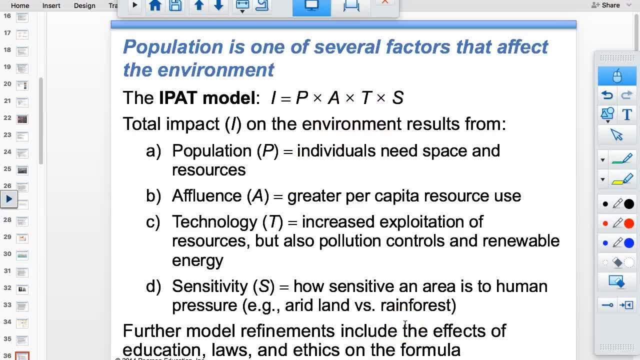 Times affluence, that's how much money we have- Times technology And then cultural- not cultural, excuse me- environmental- sensitivity. So what that means is somewhere like a tundra area where you have low precipitation rates, pretty dry and the environment is not very resilient. you know your environmental impact is going to be worse in those areas. 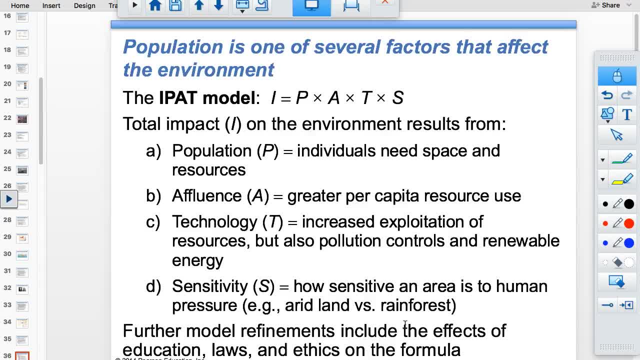 So sub-Saharan Africa, where they're in a kind of savanna sort of situation where there's, you know, not a whole lot of vegetation as far as trees. So we're starting to deforest that area, kind of the chaparral, too. 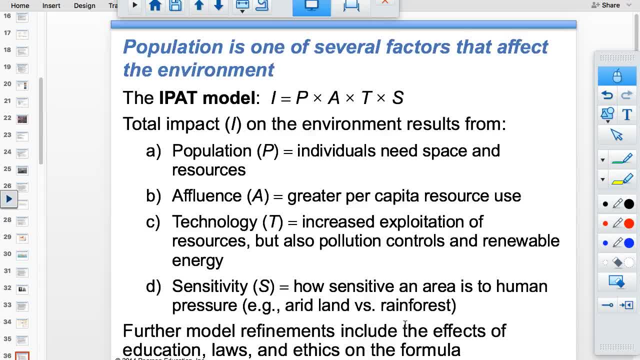 It's very pronged. It's very pronged to this, And so then you have erosion and it's not going to grow back. Vegetation is not going to grow back very quickly because it's so dry And so, unfortunately, a lot of places that we have high population growth rates are sensitive as far as the ecosystem that's there. 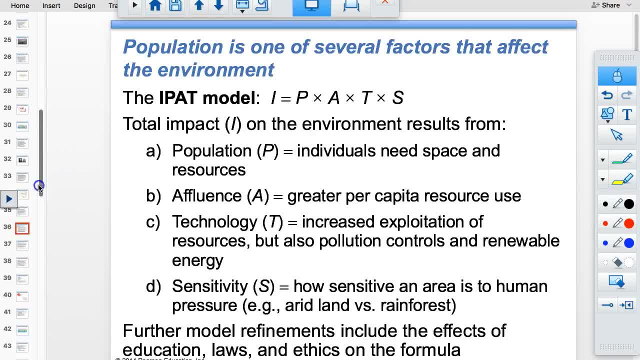 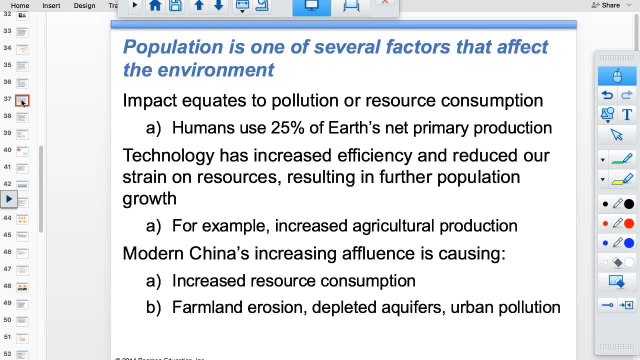 No worries, though, right, Everything's fine, It's totally fine. So there's your nice little formula. You don't actually ever put numbers into that. I'm just going to school that for you. So, as far as humans, we're using 25% of the Earth's net primary production. 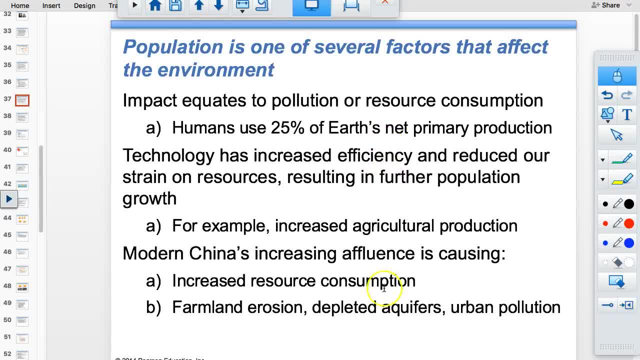 So net meaning, After the plants get done, doing respiration, Remember this, Okay. And so that's obviously through agriculture and then us feeding our livestock. So technology has really increased our agricultural production. It's what's led us to be able to be at 7.5 billion people. 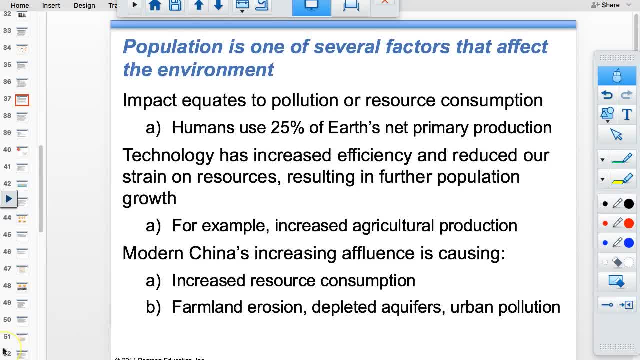 And so now we have this problem with these developing countries and they're starting to become more affluent, And then they're wanting to be like us because we're so cool. It's a terrible idea because we're so happy. Never mind, we're not. 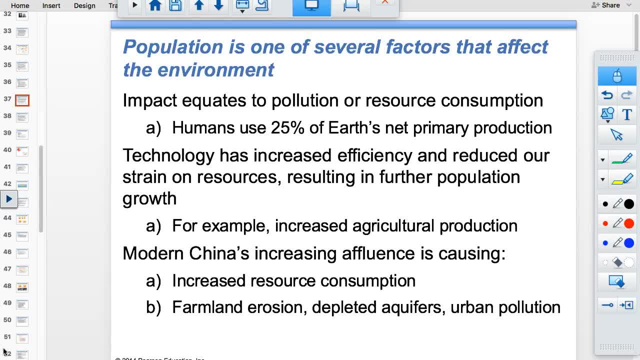 And so, as these developing countries want to become more affluent, that'll be good because their birth rates will go down and their population will go down. But then what is our ecological footprint compared to theirs? Scary, I find demography to be extremely interesting. 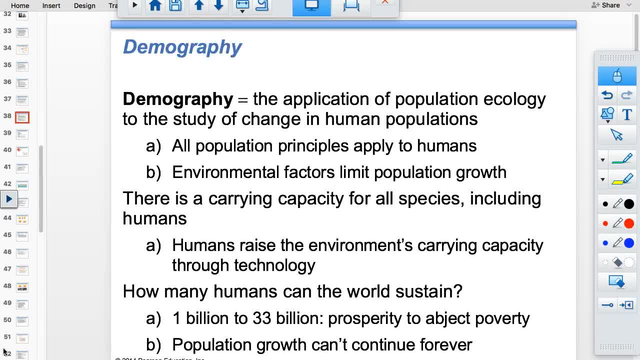 I took a human geography class, a demography class, in college. before I even knew I was going to teach this. We learned about population pyramids. It was like the coolest class ever, And then my professor was the one from Canada that had gotten paid to have four kids. 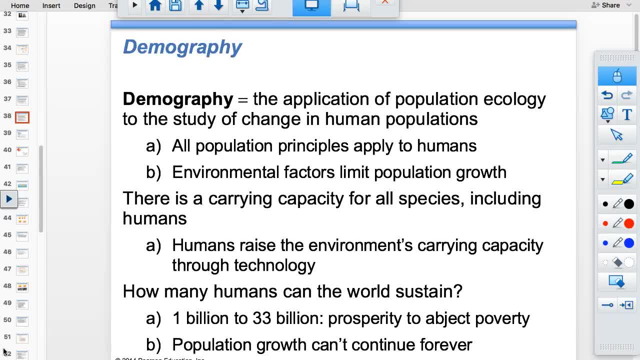 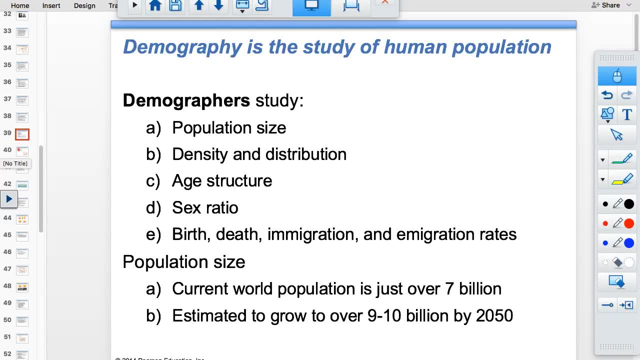 So it was like A lesson in a lesson, Okay. So, anyway, studying humans and how we have raised our carrying capacity through technology and all these population principles, That's, demography and size, age structure, sex ratio, density distribution, all these things. 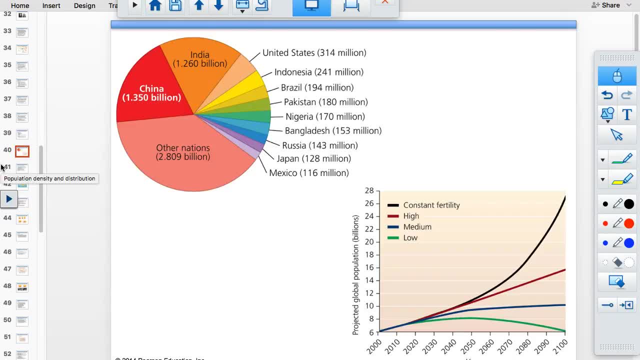 So I think this would be a cool job, by the way, But I don't get out much. So here, most populous countries: China, India, United States and then Indonesia. We already talked about that, You sure you know it. 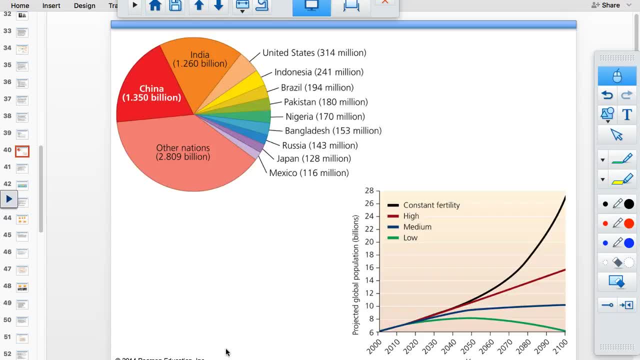 How you feeling? Okay good, And this is terrifying. If we keep our fertility constant, we'll be at a whole 26 billion by 2100.. Anybody plan on living 83 more years? Just let me know how it goes. 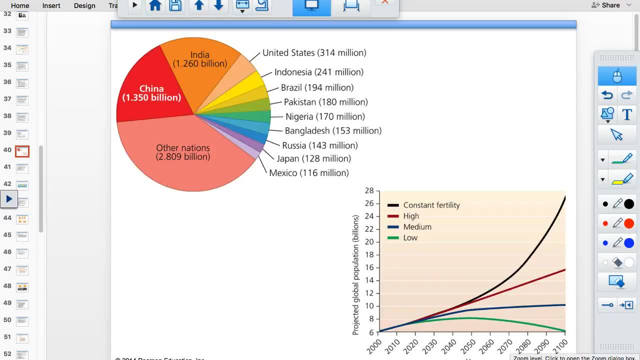 I don't think I I might live 83 more years, But you might. You would love to be 100. You'd be really crowded. Our population growth rate. fertility shouldn't stay the same. It's kind of impossible for it to. 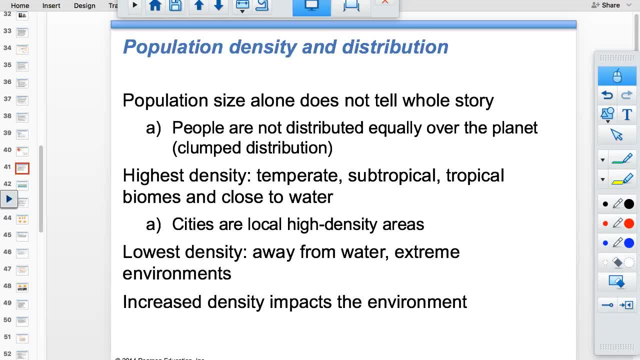 Science doesn't tell the whole story. It turns out that we are not uniformly Distributed as people like we're clumped. if we were fish, we'd be in a school. We actually are in a school, but we're not fish. Okay, I'm on fire. 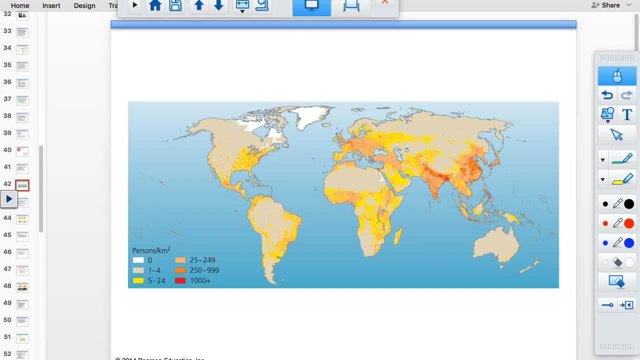 So if we look at this and you can see that as far as where people live, they- if I draw the equator above the part of Brazil, that's my fancy way of saying it- we have people mostly in tropical and subtropical areas and temperate areas. 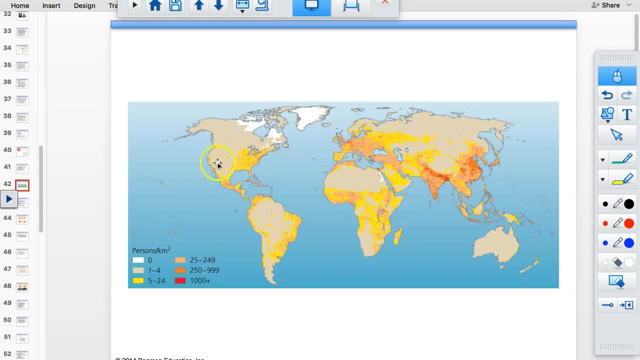 And so here's the East Coast of the United States, there's the Rockies. We're like- no, I feel like going to this just like how America is, And so India is very crowded. Here's the Himalayas, And we have to go be desert going on. 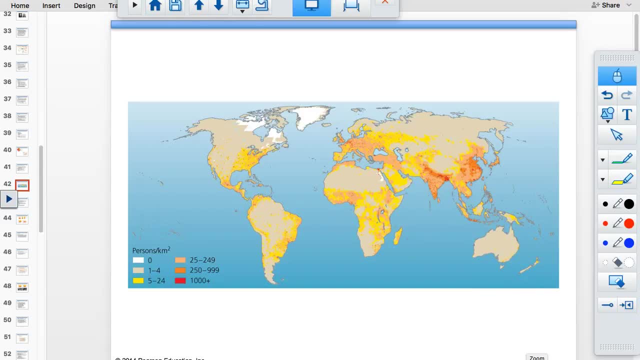 Australia is just a big desert. It's at 30 degrees south Live to 30 degrees. It's kind of like, hey, here's a desert, So yeah, here's rainforest. There's like that one tribe that lives right there. 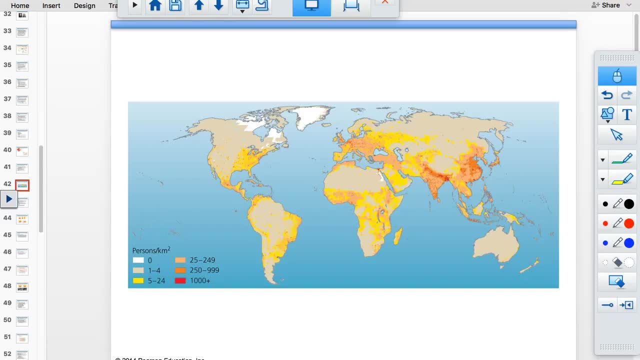 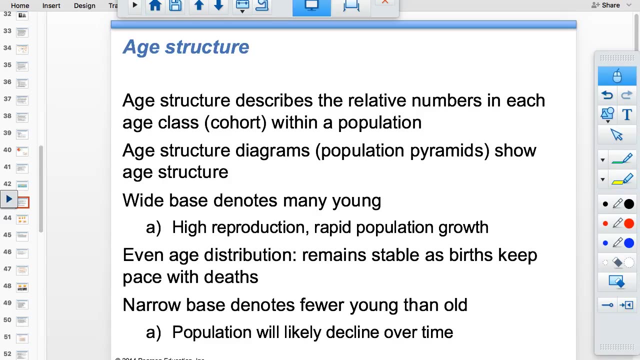 I'm kidding, So you can kind of see that we're- we're really big, clumped along coastlines and then, in pretty nice climates, a structure diagrams. We're going to look at those. There's five or six questions based on these pyramids tomorrow which I hope you feel OK with now. 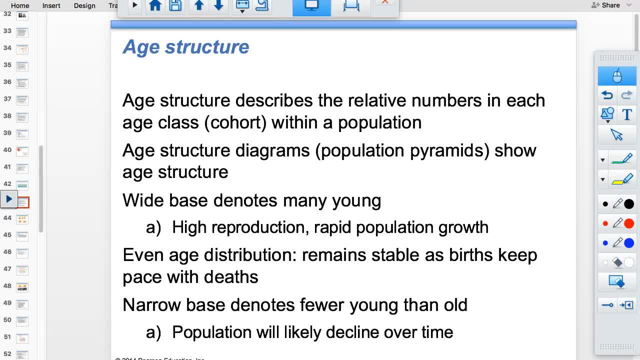 Each structure describes the relative numbers in each cohort within a population. You cannot ever get away with saying that the bottom of the pyramid looks like a pyramid And so since it has a wide bottom, then it's going to have. No, you have to say that the pre reproductive cohorts are larger in number than the reproductive cohort. 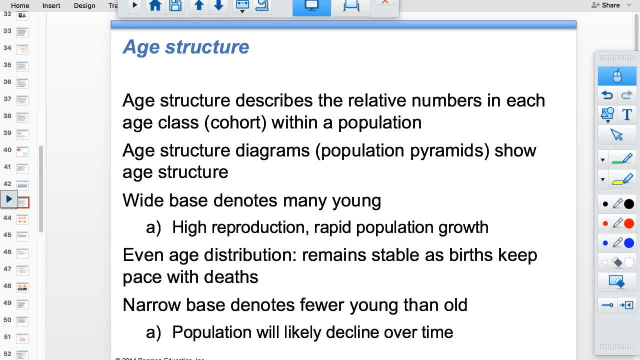 So the total fertility rate is higher than replacement, Like those are the things you have to say. So, as you're studying for your ever, If you look, I'm pretty sure that's one of them- as population pyramids- Make sure you watch how you say things. anyway. 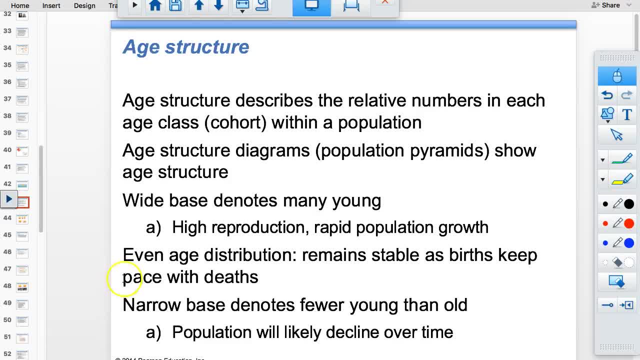 So an even age distribution, That's where we have the same number of individuals in each cohort until, I mean, once you hit 60, they're all going to go down, because people do die eventually. We can tell that that's going to be steady. 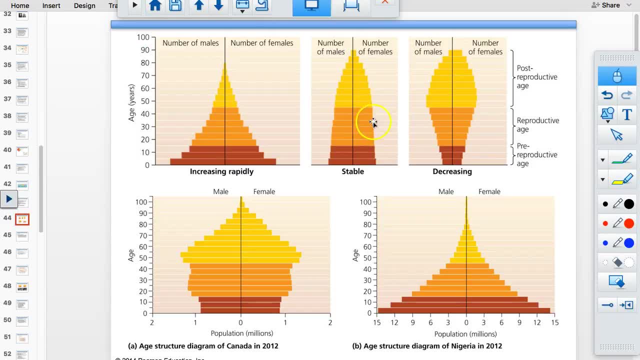 So what I was just trying to tell you is here. you know, once you hit 70 or 80, they are going to decrease, because people do die, But this is stable. This is increasing. Let me say it to you one more time: how to say the things? the pre reproductive cohorts are larger in size than the reproductive cohorts, which indicates that the population is above replacement as far as fertility. 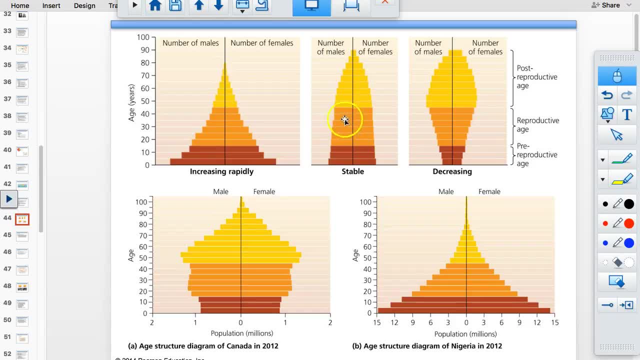 And when I say replacement fertility, that means that these people are having the just enough children to replace themselves. here, with decreasing, I can see that the pre reproductive age is lower than the reproductive age cohort. So the people pre productive age in this country actually have a lower fertility than needed to replace themselves. 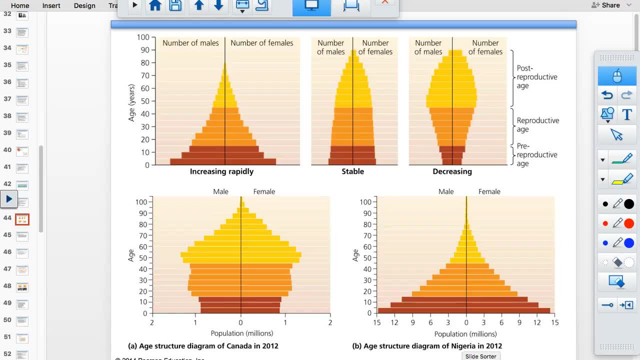 Can you say the magic words? Okay, good. So here's Canada in 2012.. And you can tell that my professor was paid to have children, right? Canada has a negative population growth rate. And so here's Nigeria. Don't think they're paying anybody to have kids. 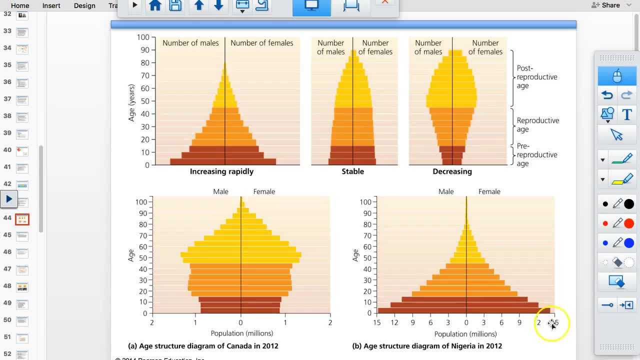 It would look like that, But this is. this is quite drastic, and you can tell too. you can get information about quality of life. as far as we can see, the age expectancy here is really starts to decline pretty steadily after 50,, 40,, 50.. 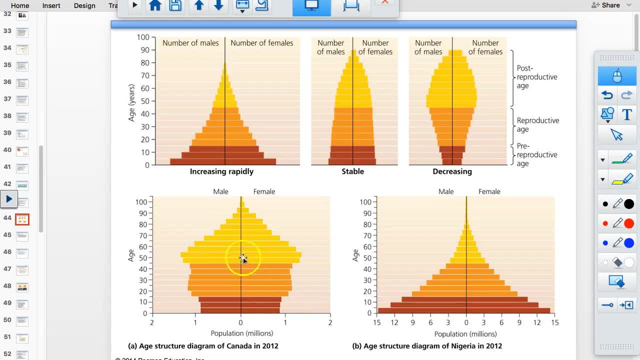 So that's not really happening in these other pyramids until 60 or 70, kind of see what I'm talking about. So it's not only just growth, growth You can look at. you can kind of get some details on life expectancy as well. 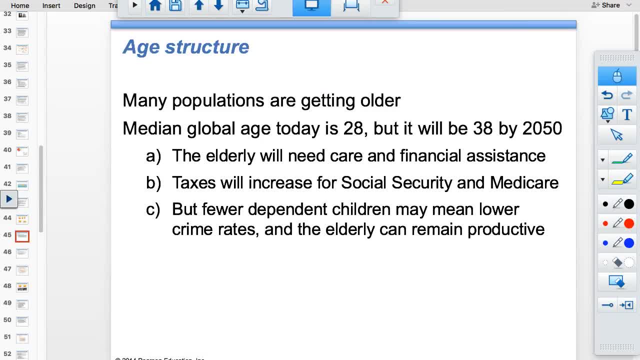 All right. So populations are getting older. The average median global age right now is 28 and it will be 38 by 2050, which is good, but absolutely need care and financial assistance. So even if we slow down our growth and stop having so many kids, who's going to take care of these people in their old age? 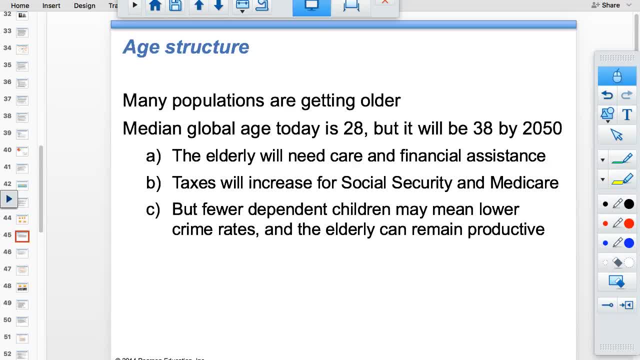 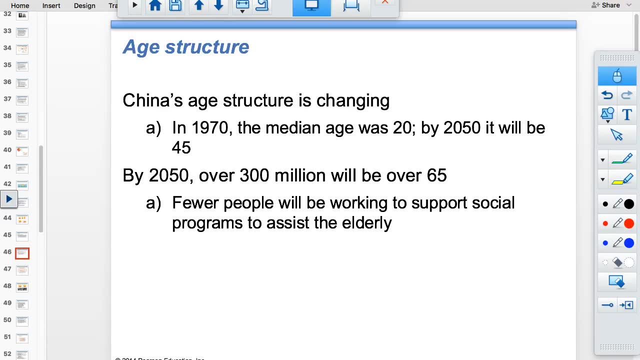 Okay, Fewer dependent children. Children do cost a lot of money. School costs money And then just typical deviant youth hood life. that costs money and as far as crime. So you know. anyway, China is is changing. in 1970, when they started the one child policy. 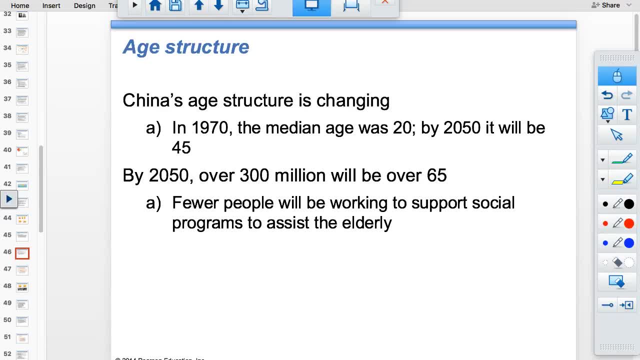 The average age was 20 and now, or by 2050, would be 45. So that's- this is terrifying The whole population of the United States in China, like that, many people in China will be over 65 in 2050.. 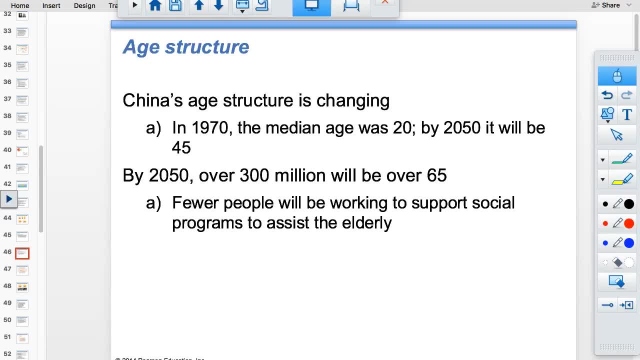 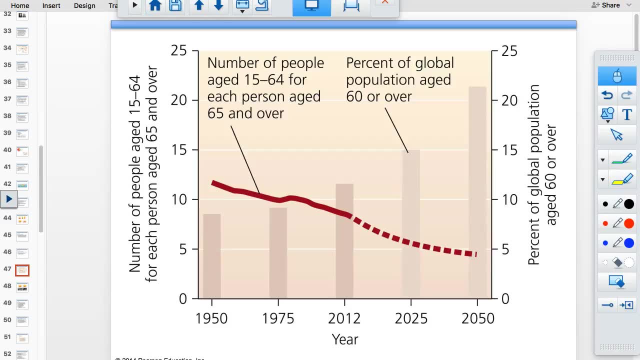 So they're going to have quite a financial burden to bear, And so I really feel like that's why they, you know, say, okay, well, I guess you have two kids now. So anyway, the number of people: 15 to 64 as we go through. 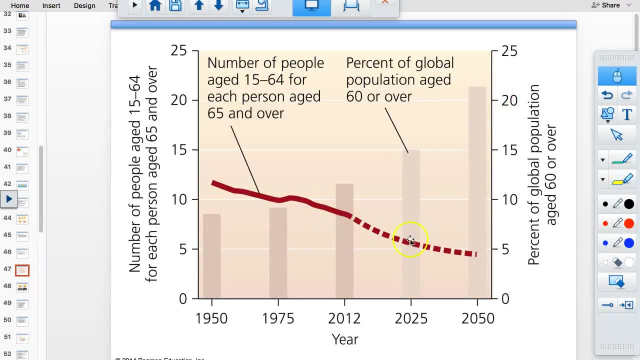 that's going to go up, right? So this bar is showing us that the number of older people is going to go up, And then the number of people that are 15 to 64- is for each of them is going down. So you have this red line shows like basically productive members of society. 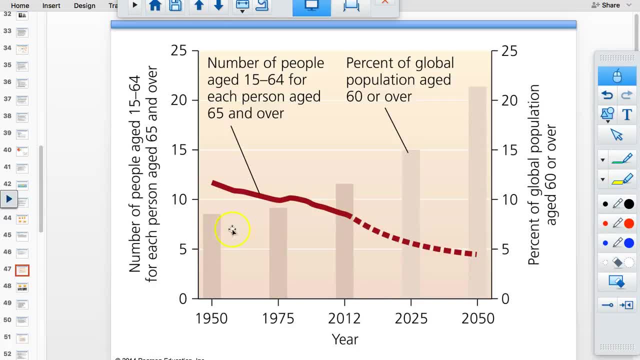 15 to 64.. And then the people that are 65 and up are going to be going up this year or each 25 years. So I don't know about the scale of this graph making me question my life, but whatever you want to do, 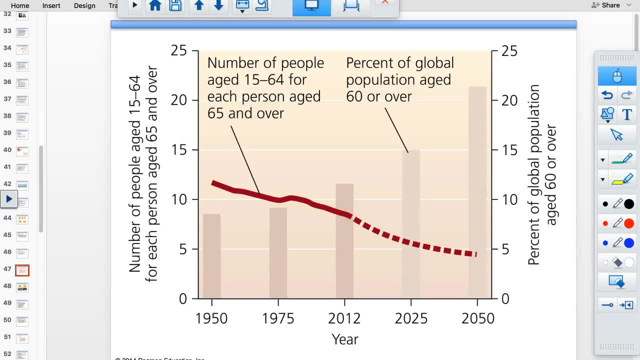 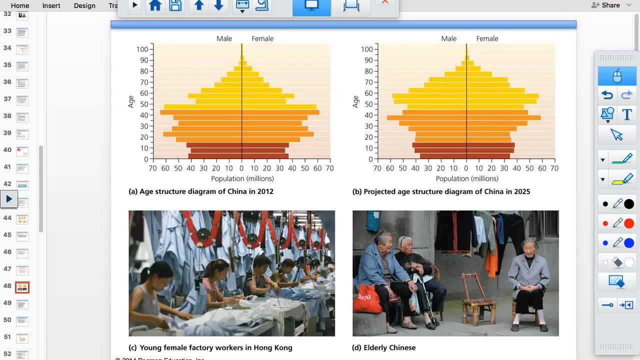 textbook. I like every 50, 12.. Never mind, I give up. Okay, so let's take a look at the actual population pyramid for China, And so I really like this. If you can see, you can see the idea of population momentum. 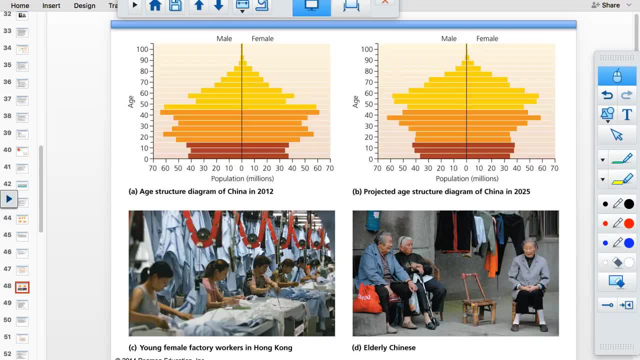 Population momentum. quite well, So check it out. If they started there, if this was from 2012,, okay, and they started their one-time policy in 1970, then we would expect to see a decline in fertility about around the cohort of 40 years old. 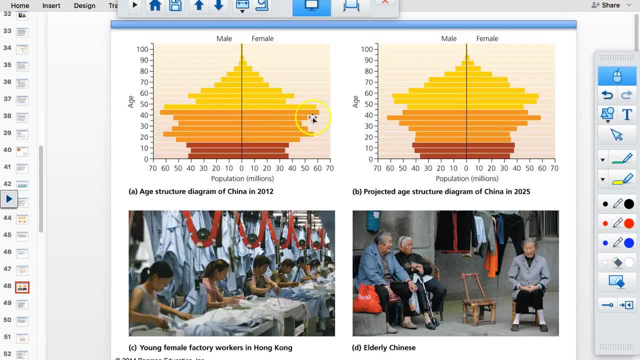 So we find 40 years old And then I mean immediately see the decline. Can y'all see that? So this is where the policy started. And then we start to see the decline in the number of people, right? So 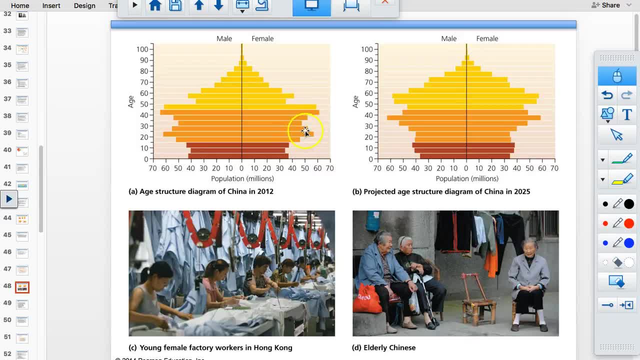 well then, what's this about? See, this little, what this is called, is like a. it's like a baby boom In the United States and European countries and Canada, where they- well, Canada was really as much with World War II. 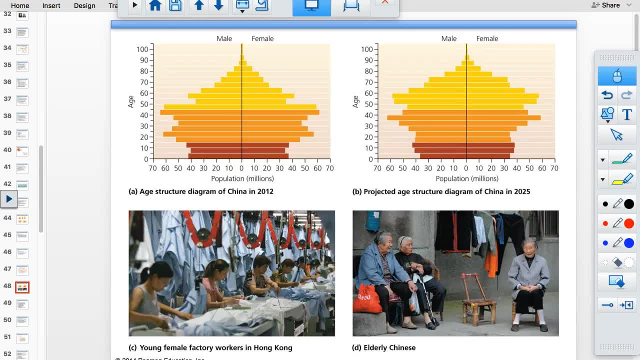 but European countries and the United States. we have a baby boom around this time post-World War II, And then you have what's called the echo boom. So you have this little, last little bit of people that were born before the one-child policy started. 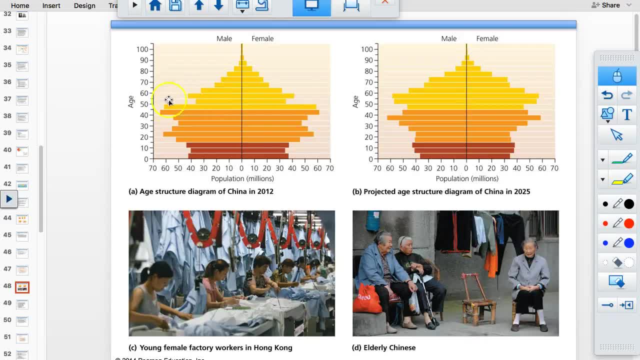 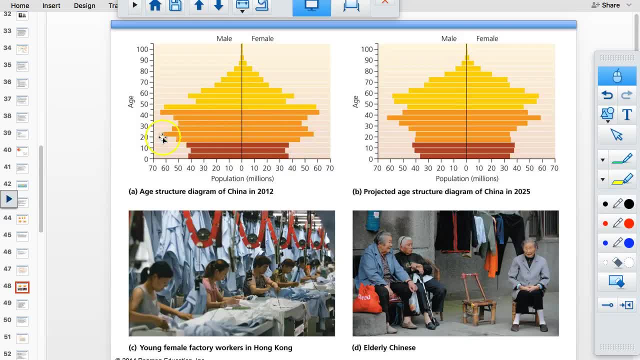 no more than one kid. you still have that increase in population growth once those people become 1997, 01'una, 00'unui, fertile. So that's the idea of population momentum, And so you still see this. You'd actually kind of follow it one more time. 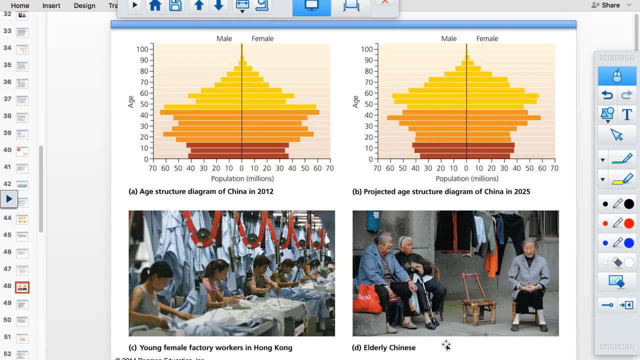 but it becomes smaller. Um, actually it's not there because I don't have one kid, so, But you can kind of see it takes a few generations before we actually stabilize the base of your pyramid. you really, you see that negative growth, so, um, you can just be. 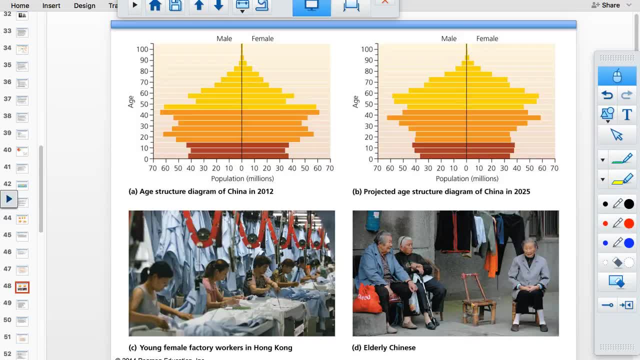 happy. i don't know what they're doing. they look so happy. they're chilling out. i think it's great to be in. um, i don't know. i can imagine a photographer going up to them be like, can i take your picture? yeah sure, um. so i'm gonna actually take a little break here. stop talking. 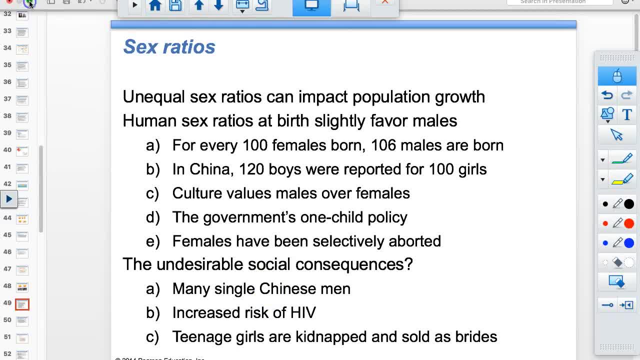 for a minute and pause my little movie, which i hope is still going. yay, okay. so sex ratios sounds like fun math, but it's not um, um. so unequal sex ratios can impact population growth and so, uh, human sex ratios, uh, at birth slightly favored males, um so 100 males to 106 males for. 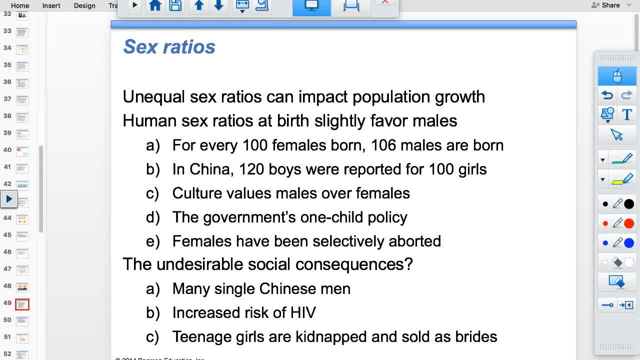 every 100 females, but in china there was 120 boys for every 100 girls, and so that was from cultural preferences and, like i said, it caused problems that we talked about before i started the lecture with um kidnapping um girls from the countryside. increased risk of hiv because. 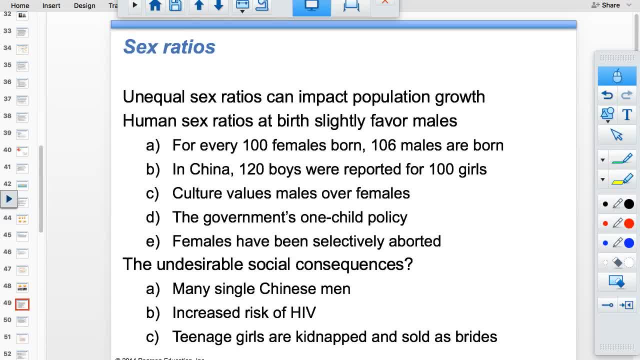 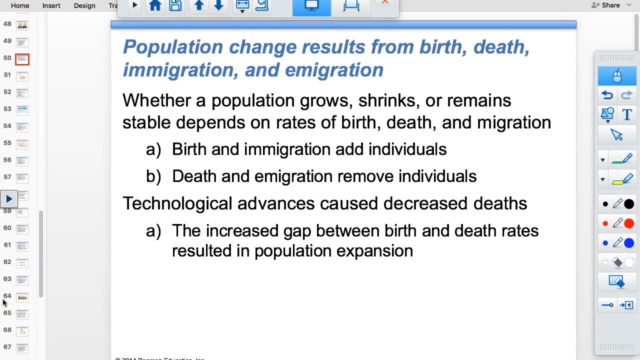 you have increased promiscuity because you have, uh, um, you don't have enough females to have monogamous relationships with every male, to understand. so, um, that's the issue there, and so you have a lot of single people and that's just, uh, the situation currently. so, whether 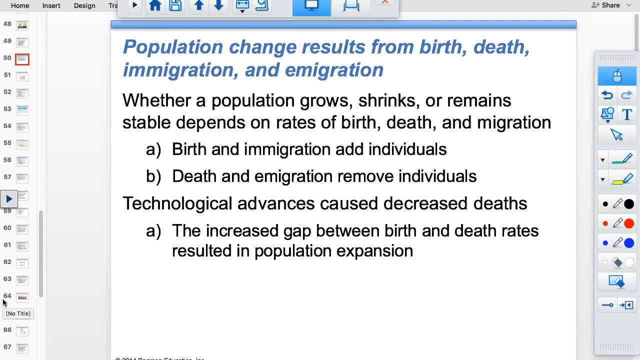 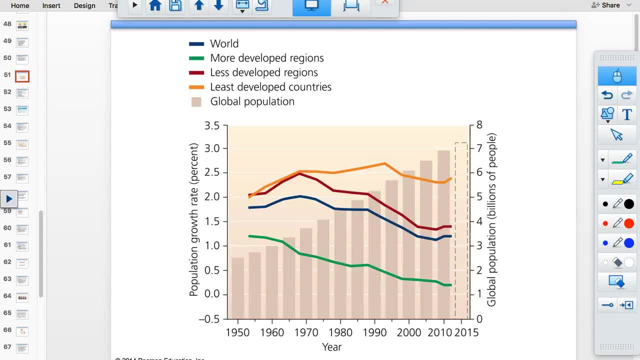 population grows or shrinks gonna depend on a lot of stuff: birth, death, immigration, immigration and then technology. so, um, if we look here again for the third time today, the least developed countries have the highest population growth rates. um, the most developed countries um actually the lowest growth rate. so you know, people are getting added to the areas. 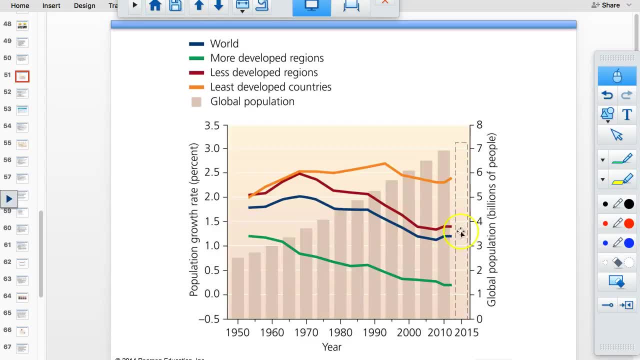 that cannot support them. and, um, by 2015, which we can already answer this question because it is now currently 2017- we are at seven and a half billion. so, um, that graph is pretty accurate. as far as you want now tfr, sometimes they'll give you those letters and they'll tell you what they mean. 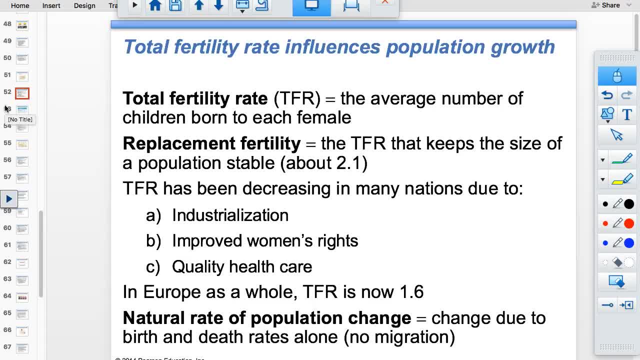 so you have to know what it means. so tfr is total fertility rate. it's the average number of children that each woman in a society or country or area or whatever is having. so it's basically: how many babies does each lady make like that's it like. you just need like an easy definition, um. 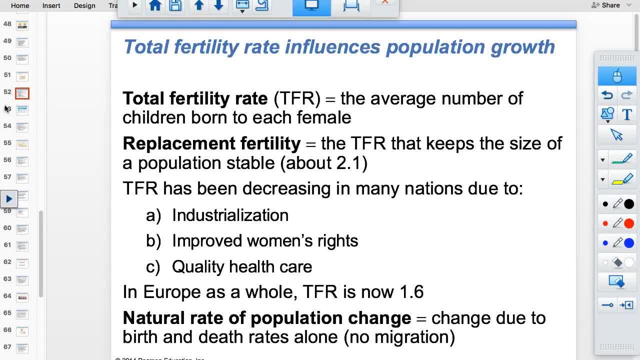 now, as far as replacement fertility, that's different in a developed country. notice, i'm not saying first world, third world, something that that makes us feel like we're winning, but we're not. you know, we're really not um so um. in a developed country, the replacement fertility 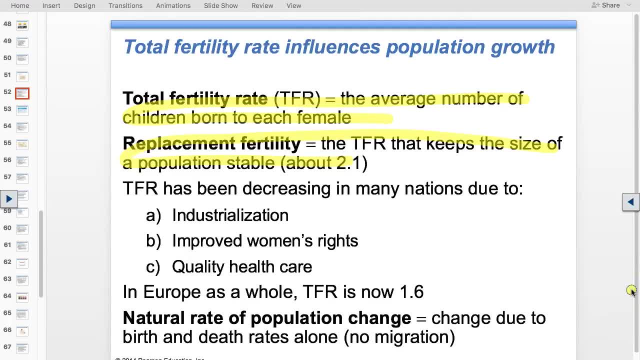 is the number of children to replace um the parents, and so it's 2.1. you would think of b2, but the 0.1 is an average. that's because it is an average and it comes from the fact that some people don't choose to have kids, or they're infertile, or they don't survive to adulthood. 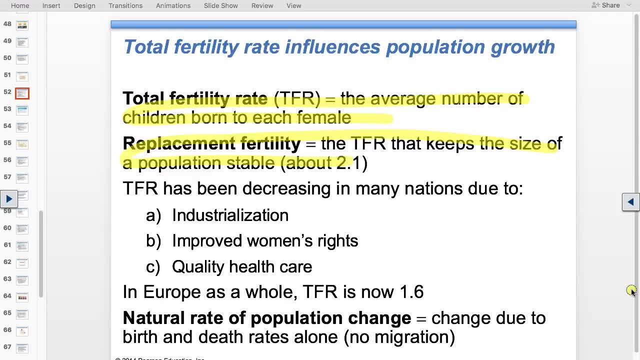 or whatever, um, and so your tfr has to equal the replacement fertility in order for the population to be stable. the replacement fertility in developing countries- developing countries- is around 2.6, and the reason um it's higher is because you're going to have problems with infant mortality. 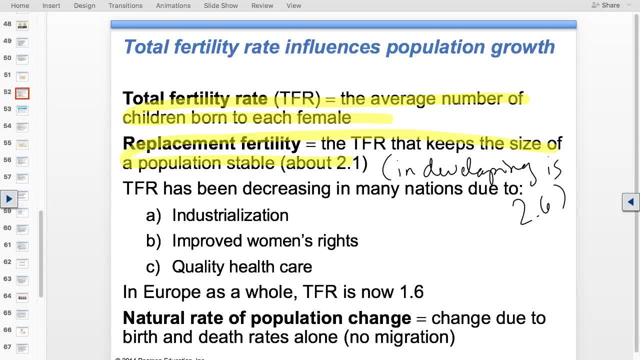 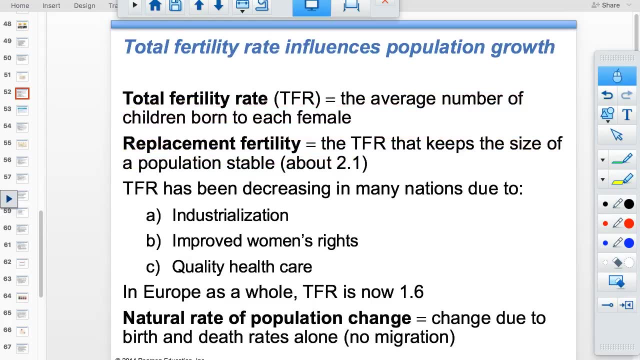 because lack of medical care for the mothers you're going to have problems with clean drinking water or childhood diseases due to dysentery- just simple things that immunizations can fix, stuff like that. um, so tfr has been decreasing in a lot of countries because of the increased 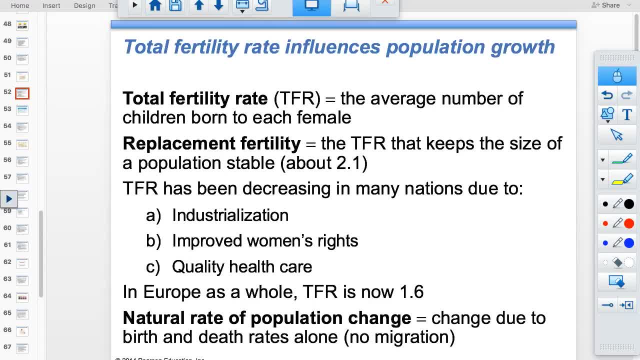 uh, women's rights, industrialization, living in an industrial society, like i already told you, it's more expensive, so people choose to have less kids because they have to pay for child care as they work, for example. um, so the number of tfr is currently 1.6, so that's much lower than the. 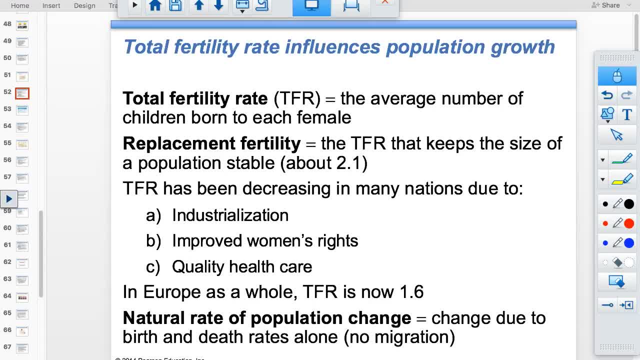 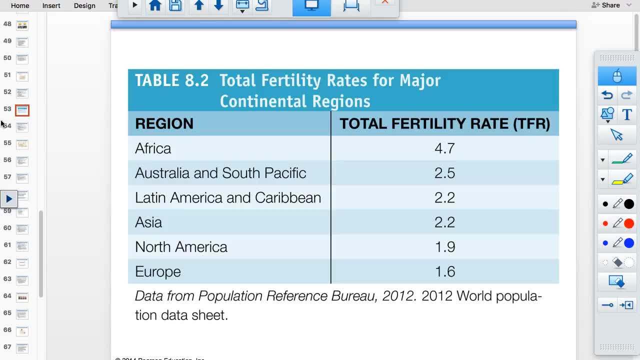 tfr needed to, you know, keep the population stable. um, so if we look at that as, uh, you can tell that the, the places that could support the children, really are not having the tfr in africa as a whole continent. africa's not a country. you don't be that kid. okay, good job. um, it's 4.7. 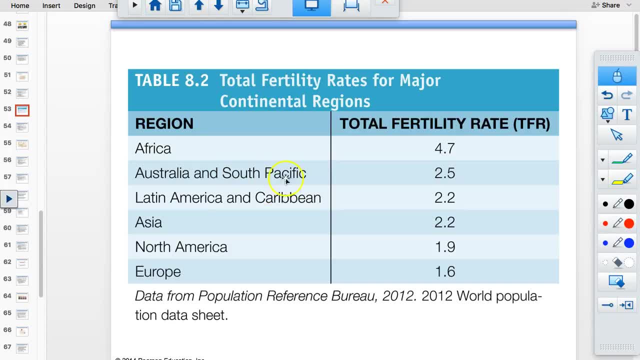 california in the south pacific. the south pacific is what is bringing up this average, by the way. okay, um two and a half. uh, latin america: 2.2. asia's 2.2. um china is bringing down this average, yeah, so um north america: 1.9, this number is being brought down. 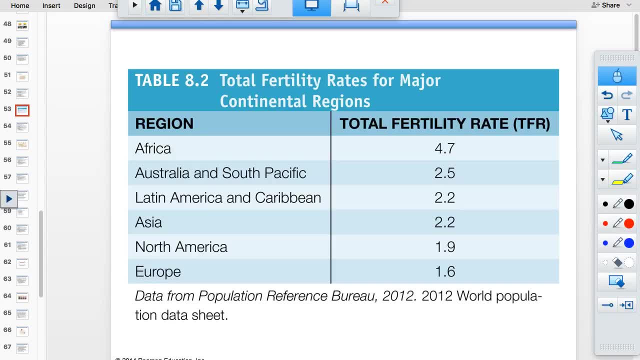 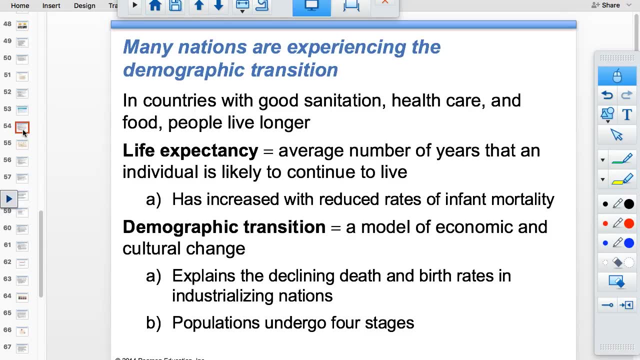 by canada um, and then europe is 1.6, so you can see a big difference there. um life expectancy, it's a good way to tell on the overall quality of life in an area. it's the average you know that you're likely to live and it does include the statistics from. 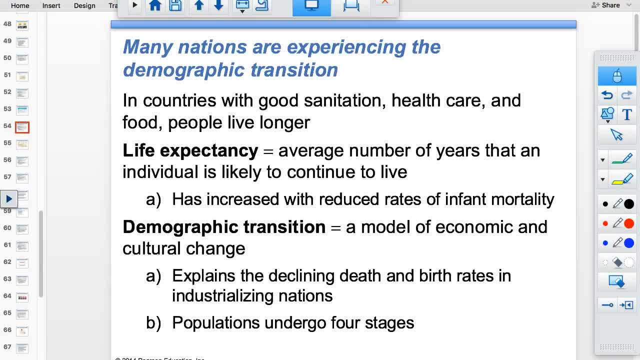 infant mortality. remember, infant mortality is death with age five. so if you die when you're three, then that is obviously going to when you average together, bring down the life expectancy in the area, so the demographic transition. I'm actually going to draw this and I'm going to explain to you as 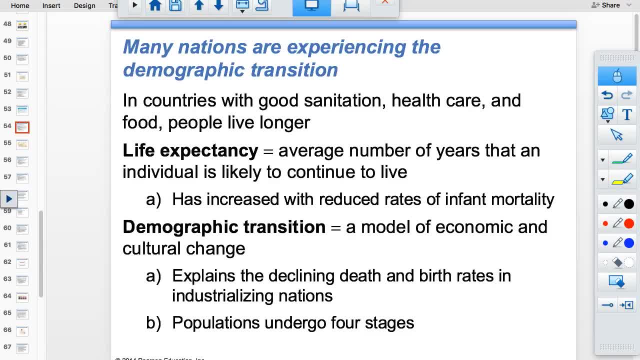 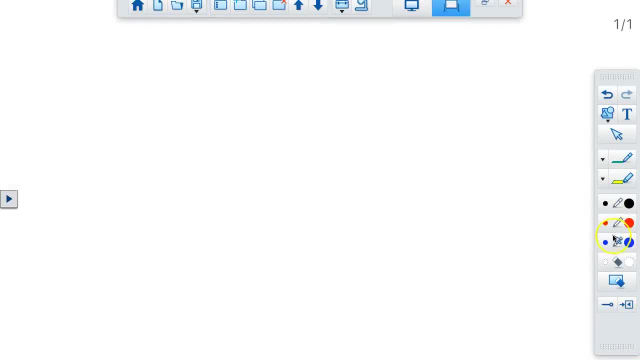 I draw it because it makes it easier to understand. so it's a model of cultural and economic change and there's four stages, okay. so, oh look, I already drew it. never mind, that's kind of sad, it's like let me do it again. so I'm gonna make the 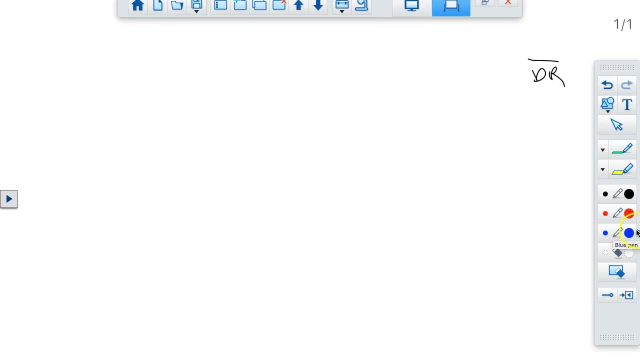 black line be the death rate, because that's just our cultural preferences, and then I'll make blue be birth rate because boys are better than girls. I'm just kidding. but traditionally, if we go back in time before the Industrial Revolution, maybe even before the agricultural revolution, birth rates and death rates were both. 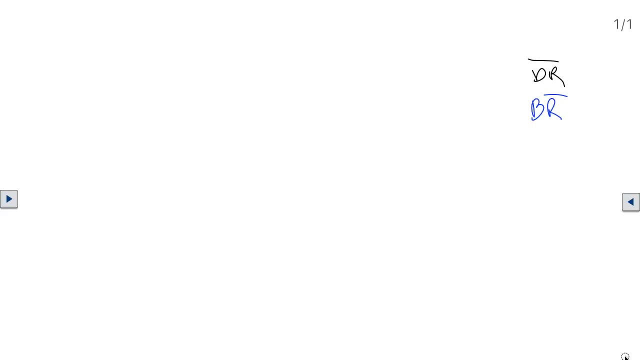 high. now they're both high. which population would grow? because you have a lot of people who are born, but people aren't living very long and your death rate is equal. so if I draw these out, I have, I have birth rate and I have a high death rate. if they're equal, right, no growth here and so for. 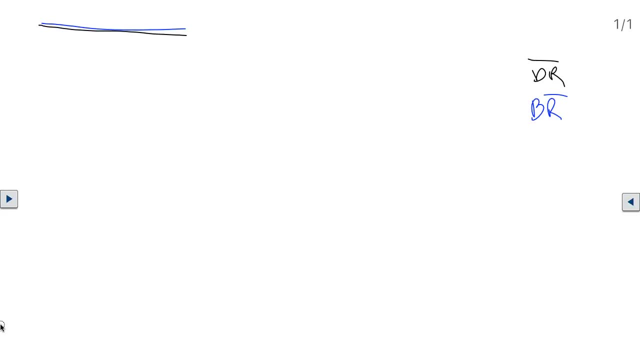 most of human society's history like that's, that's going to work now. I already told you that people will be more apt to like washing their hands and having enough food before they will give women rights, education and contraception, like that goes first, and so our ability to find diseases, increase sanitation. 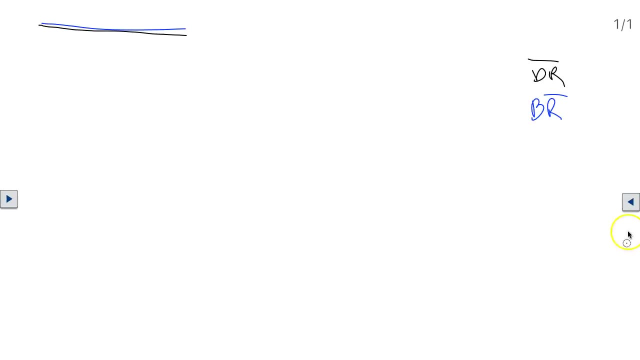 increase technology to make more food is gonna be the first change that happens. so we have four stages. the first, the first stage that I have drawn here, is the pre-industrial. the birth rate and the death rate are both high- this one's high and this one's high- so they're both high and they're equal. so if the death rate starts to, 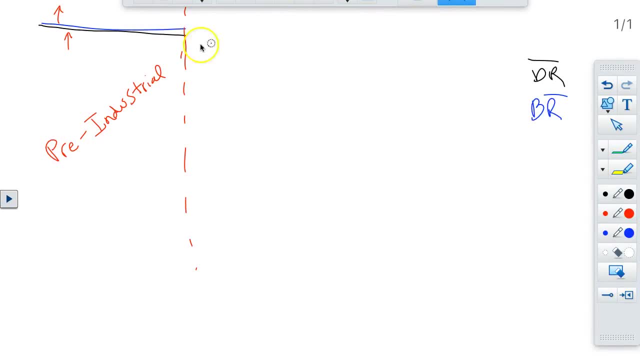 drop, because the birth rate will stay high though. so now we have a lot of people being born, but people aren't dying so much, and so this gap here- this is where we experience growth. so all this gap are people getting added to the population, and it's quick, it's very fast. this is where countries like 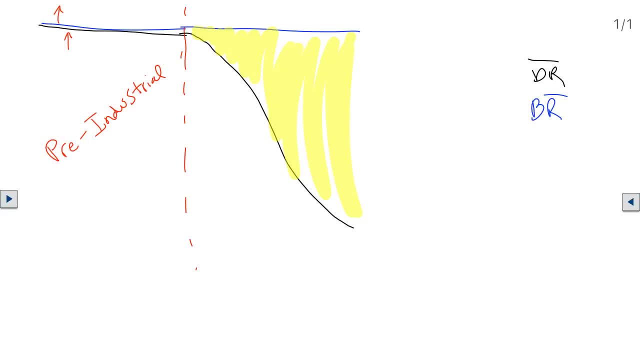 Nigeria occur. they're starting to drop their death rate because they started to have access to medical care and better agricultural practices. the birth rate is still very high, and so this is the transitional stage. now, if we had them both high, the birth rate drop. what do you think is going to drop now? 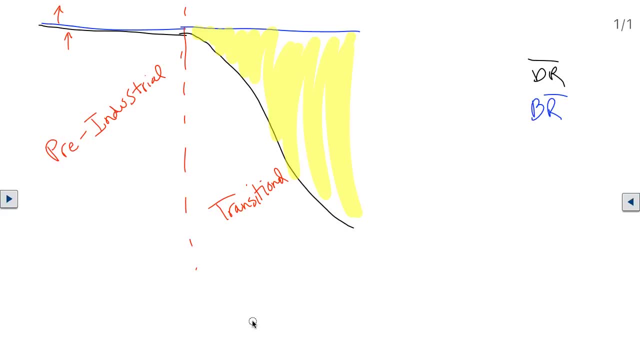 oh, the death rate. so it's really easy to kind of divide these up. I mean, it's very common sense. so the industrial phase of the demographic transition starts when the death rate drops. the birth rate is gonna stay low and when they meet they fall in love and get married. just kidding. but now they reunite here. 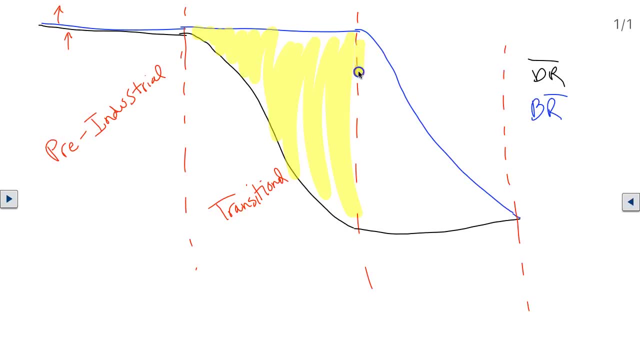 and so we see that during this period, women start to have access to educational opportunities because the society is in industrializing and urbanizing before moving to the city. the cost of having children is too expensive to have more than a couple, and then they're no longer needed for. 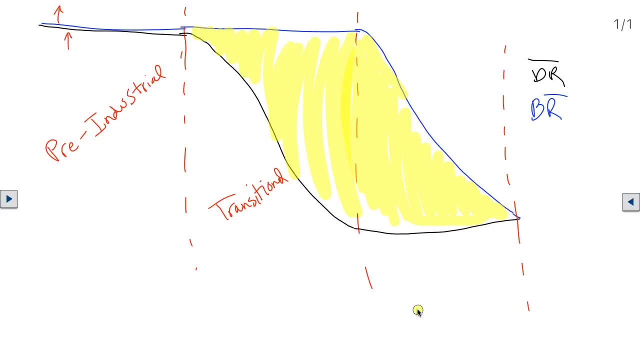 subsistence agriculture. so that's why your birth rate is going to drop for all those reasons, and a lot of that again goes back to women. so once they meet- and they're now both low- we have entered into the post-industrial and the birth rate can actually get. 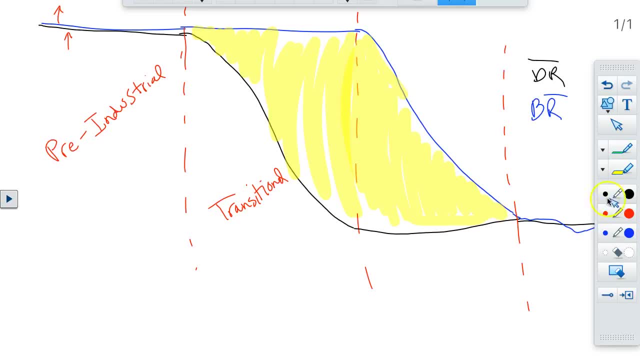 lower than the death rate, which is what's happening in Europe and Japan today. this is the industrial, and birth rates are going to slow as the birth rate declines and once they meet that's post-industrial. so if you can remember that, they both start high. people quit dying before they give women's rights. 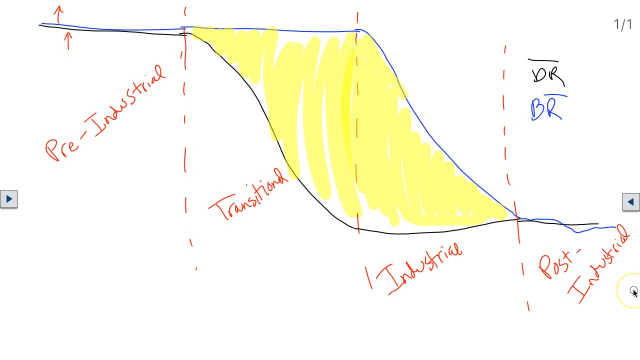 to them and they both end low. you should be good. pretty straightforward, right? all right. so the biggest question you're gonna see on the AP exam is during which phase and they'll have one, two, three, four or they'll have words. it just depends on who's. 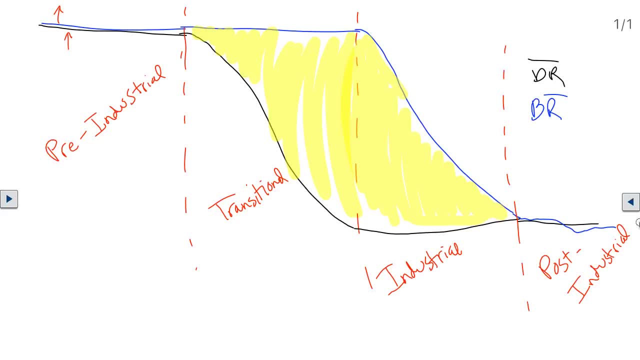 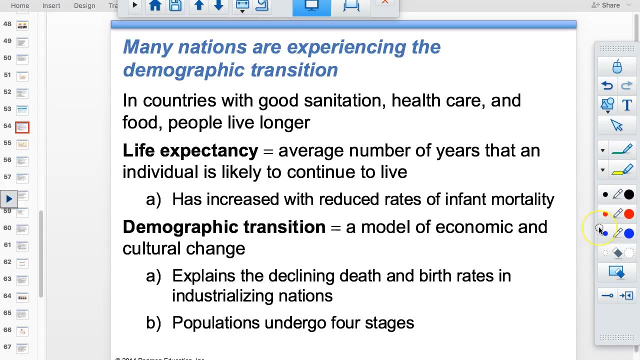 writing the question: during what phase do you see the biggest growth? and so will be phase or stage two, the transition. okay, so there's that um that's called the demographic transition. here is their picture, which maybe looks slightly better than mine, but similar. so both time: death drops, birth drops, both low. 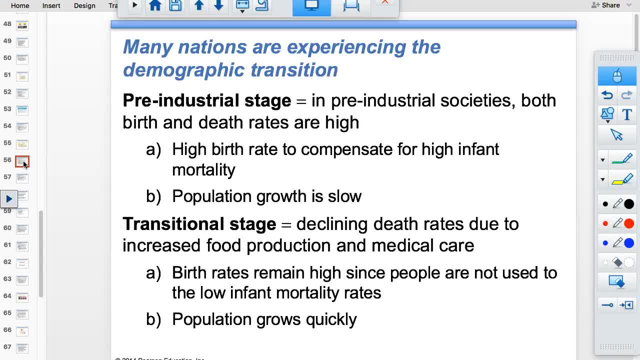 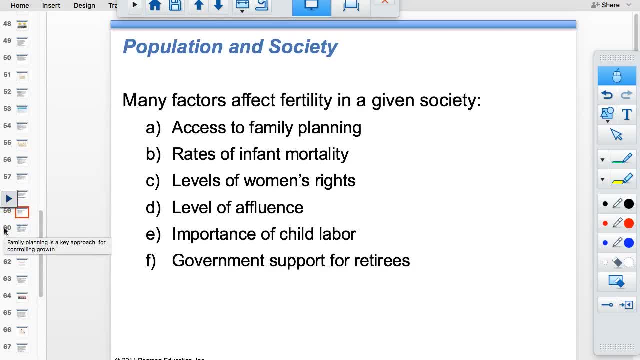 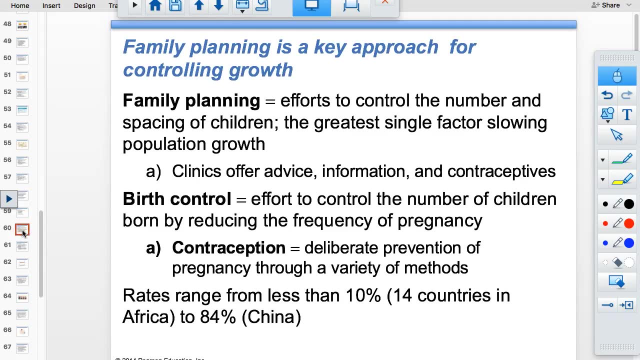 done the end: pre-industrial transition. I just explained all this and I explained it better than this. so I'm moving on with my life. fertility in a given society, women, women affluence, child labor, retirees- okay, this is very straightforward. I already talked about it. family planning can include 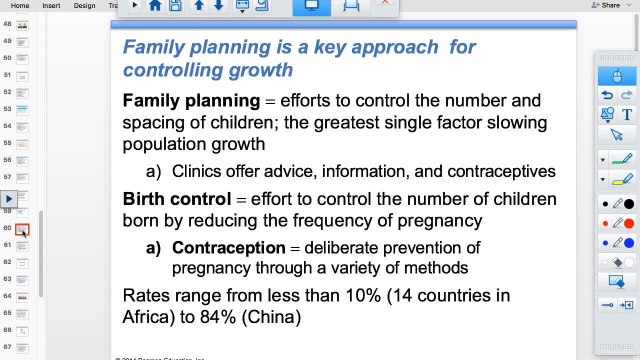 birth control, contraception- all this is on here. efforts to control the number and spacing of children is gonna be the greatest single factor in stolen population growth. so clinics to offer advice, information, contraception, contraceptives- Wow. rates of contraceptive use vary from 10% in some areas in Africa- it's not for many- to 84% in China. okay, and so China has free. 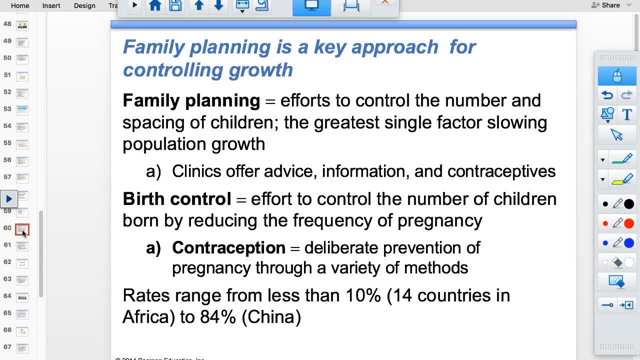 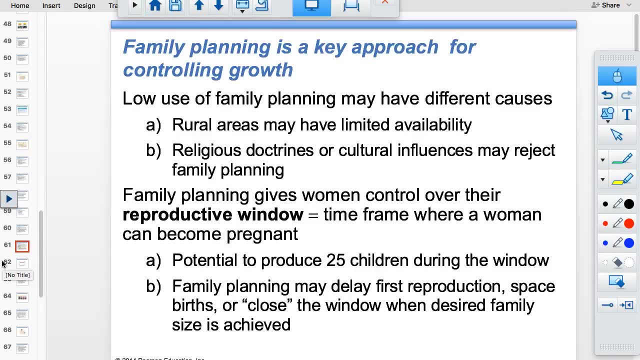 contraception, you don't mean, it's just really widely available and it costs you nothing. and so they see it as a good investment in their future as a country, because the cost of condom is much less than the cost of like a kid turned out. so just simple math there. low, low use of family planning has different causes. so 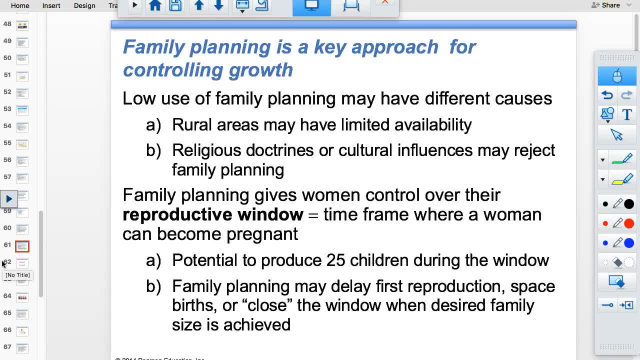 rural areas may not have available availability. so we saw in that film that I started showing you about the woman in Ethiopia that had to walk to the capital of Addis Ababa. yeah, okay, so you know, the country of Ethiopia has less obstetricians than you know, Metro. 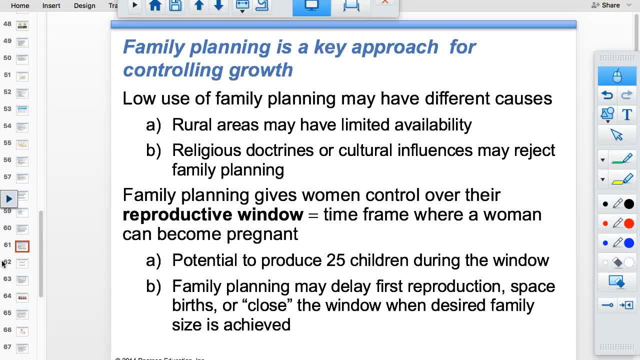 Atlanta and they have 70 billion people, million people who you need to grow really quick there. they may not have that available to them and then also some religions may reject family planning. so certainly some people that practice Catholicism don't- like we saw in the documentary, they don't choose to use 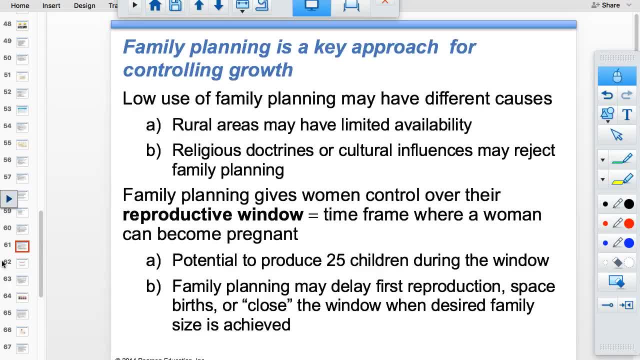 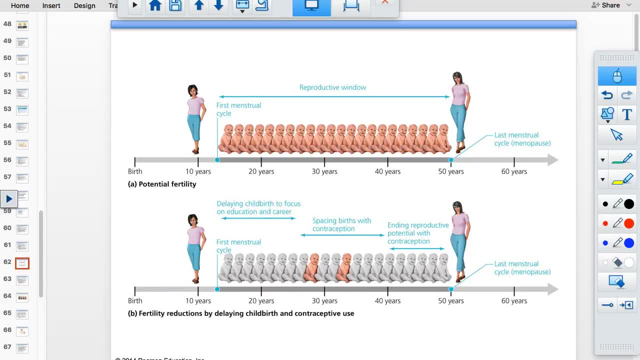 contraception, or it could be that larger society as a whole just forbid women from making those decisions. so, anyway, this is the creepiest picture I've ever seen in my life. all these little gray babies are the babies in heaven, but this diagram that I refuse to look at is so creepy. so this could be like common-core math, or like 4, 8, 12. I'm just kidding. 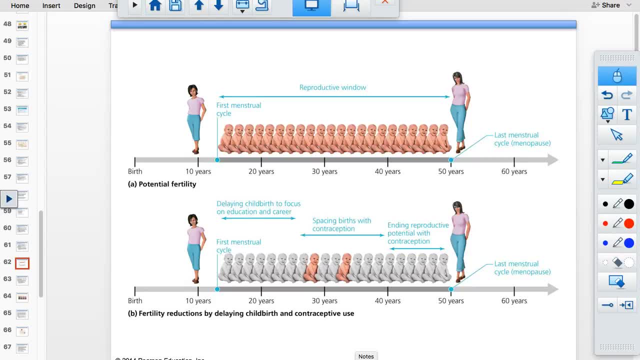 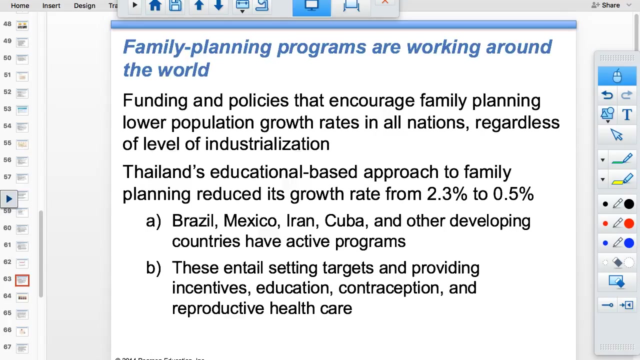 um, oh. so this shows the woman's reproductive window and basically her biotic potential. going back to that word I told you about a minute ago. and so having contraception really lowers the amount of children you have because it closes down that window and it okay, just the not okay. next. so education to people especially. 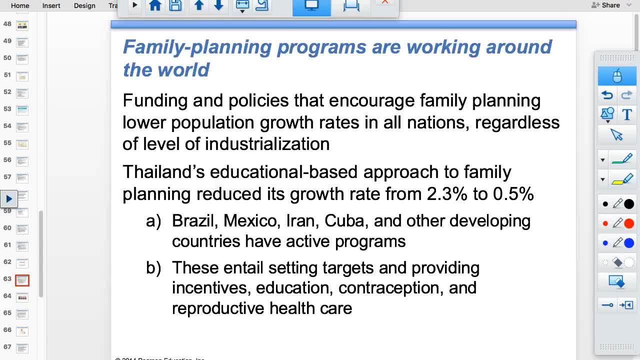 in rural areas. I mean, you saw in our documentary how people really didn't think that birth control is effective, or it was available, or they didn't think that their spouse would approve of it. and so there are these community-based educational programs in countries like Thailand that have done really good jobs. 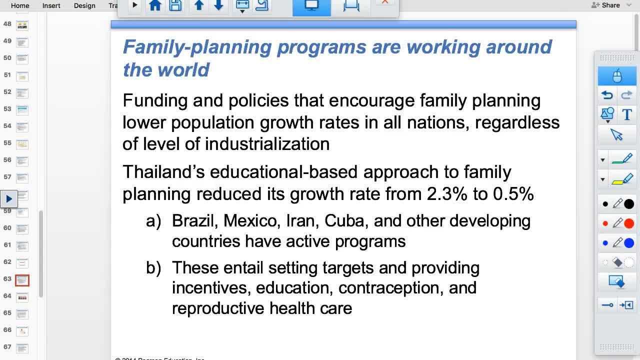 of reducing growth rates. I'm two point three percent, so you're looking at a population double in every, you know, 20, 30 years, 25, 26, point six, seven, is that it? I'm just kidding somebody, good man. and to what? seventy about? about point 5 and 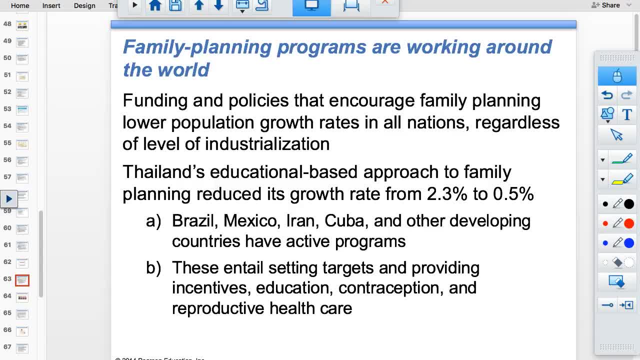 to what? 70 to about about point five and is 140. and if that's like witchcraft that I just did that math that fast, you know, half of 1 times 2 is 140.. Anyway, we've seen that Mexico's population pyramid is. 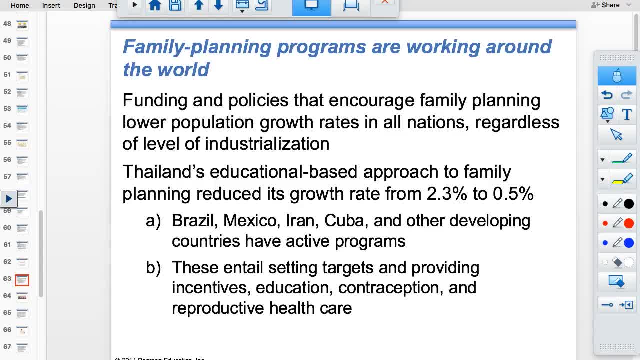 pretty stable and we can tell that the cohorts of the pre-reproductive age are similar to those of the reproductive age. We saw that yesterday in our population pyramid activity and so they have these active programs for community education and the how to use contraception. So you can see in this diagram what they've done. 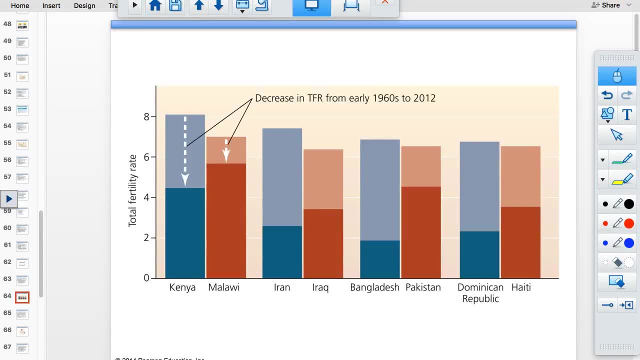 is they have. as far as culture and location, they've paired up countries. The country in blue was the country that had community-based education programs to show and, you know, tell people about how contraception works and its value and made it available to them. So Kenya, Malawi- see that you know Kenya's. 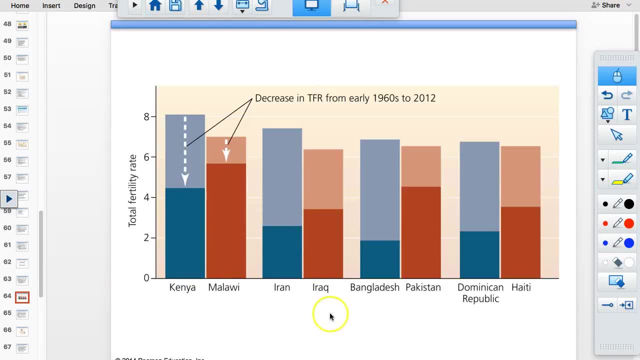 population shrunk more than Malawi's, Iran, Bangladesh and Dominican Republic. they all had you know similar things. and then Dominican Republic, really their TFR went from you know six, almost seven, to you know 2.2, 2.3. so right up replacement fertility, I mean that's. 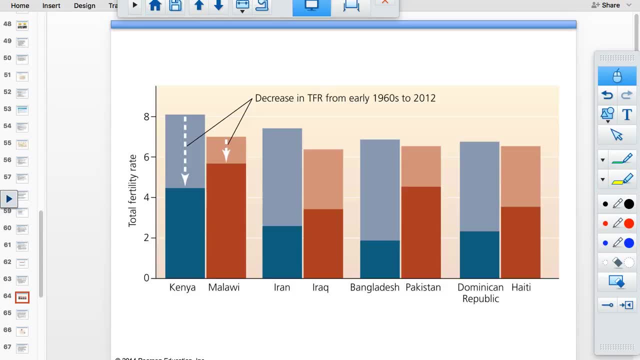 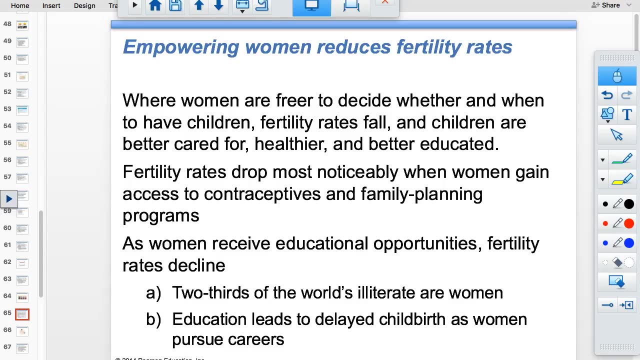 that's impressive. that's just, you know, over 50 years. So, okay, I think we get the idea about women, and when women can decide how many children to have, they're gonna be better cared for, healthier and better educated. Fertility rates are going to drop when women gain access to contraceptives and family planning. 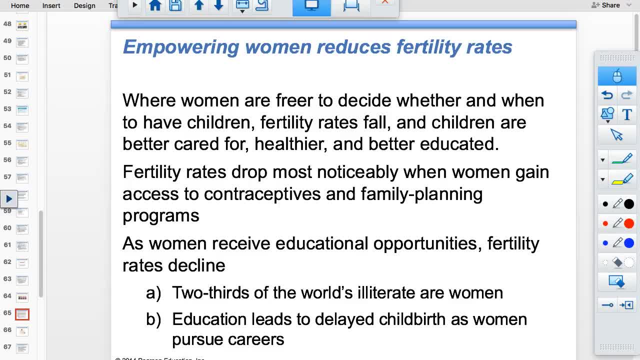 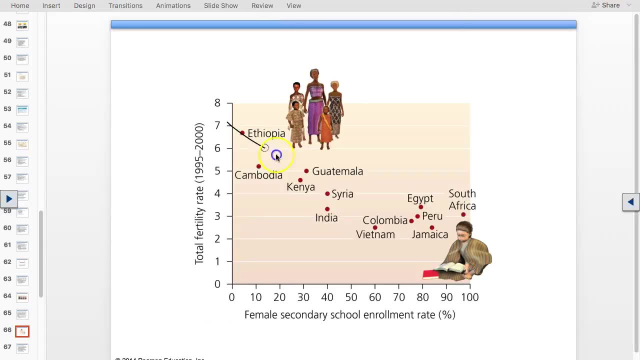 So when women have educational opportunities, fertility rates are going to decline because women are now becoming active participants in the economy and childcare is expensive- Trust me on that one- And so you can really see this really well here, and we just kind of draw a line there. This is: 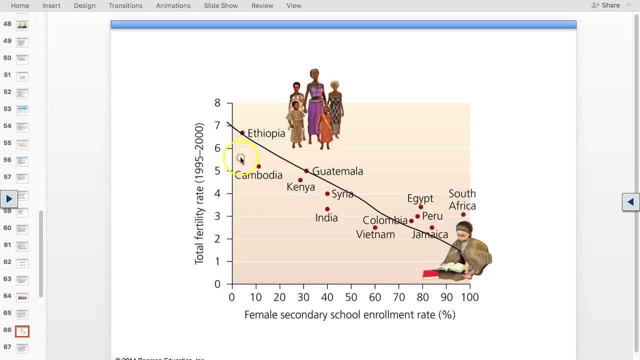 female secondary school enrollment rates, and so Ethiopia. it's over about 5%, and so the TFR is 6.7.. So if we go up here to Jamaica, where you know we have about 80% of girls in school, your TFR is closer to 2.3. So I mean it's, it's not. 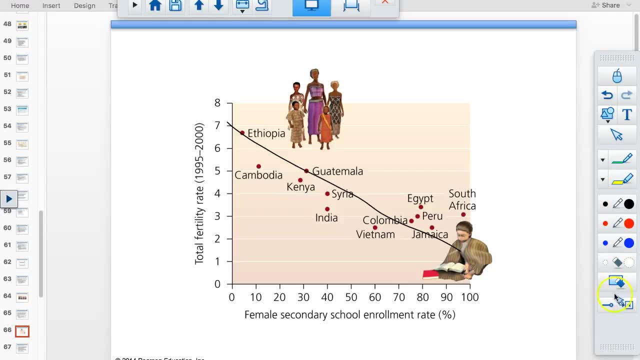 rocket science. I mean, it's very clear how those things are correlated. and so if you have lower TFRs that are higher for secondary school enrollment rates and those are correlated or indirectly correlated, Math class, Can you tell? I like math. Well, it's helpful to know how math works. 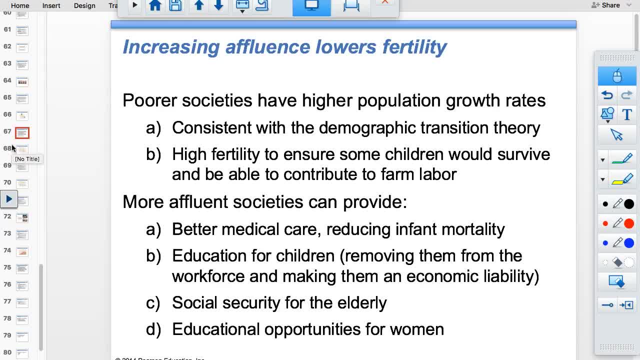 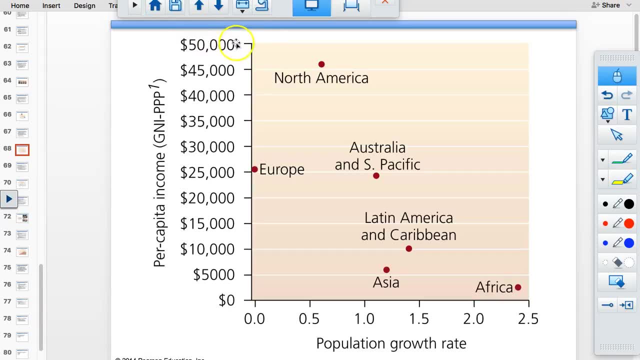 Four societies: higher population growth rates. More affluent societies have better health care, and so these things are helpful to drop in the birth rate and the death rate. So here we can see, the affluent countries. This is more money, more money, lower population growth rate, and so we're going to have that. 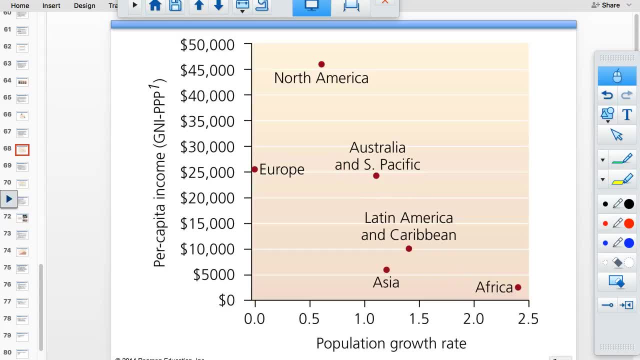 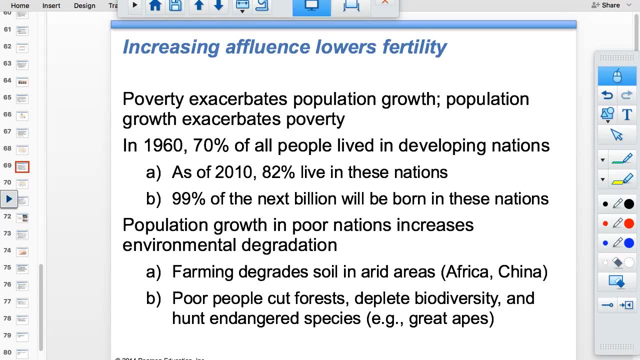 negative slope again, which shows us that they're indirectly, you know, related again So kind of terrifying. Poverty exacerbates population growth. I've already talked about this. That makes four times Population growth rate in these four countries. increases environmental degradation, especially in arid areas. If you have deforestation, you're going to have. 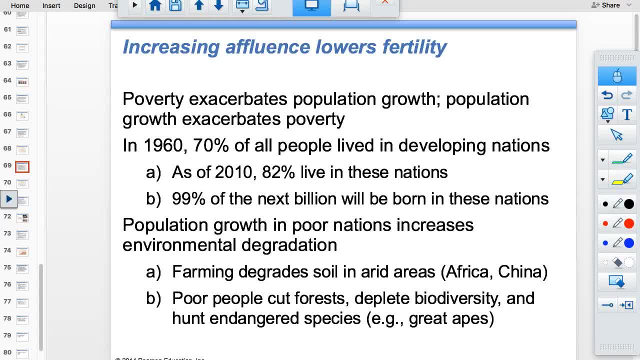 trouble growing that vegetation back. So four people cut corn, clean biodiversity and hunt endangered species. You know we get older. you know they're taking people on lion hunts. Poor lion, I'm sorry. if you had 6.7 children and there was a lion in your backyard I bet you would go hunt it so you could. 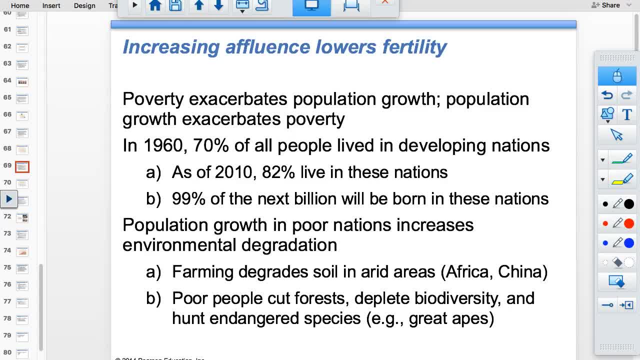 feed your kids, Don't you think? Yeah. So, like I said, when you look at these international issues, you really have to ditch your personal perspective and kind of take a mile in their shoes The way they don't have any. So, yeah, Okay, moving on. 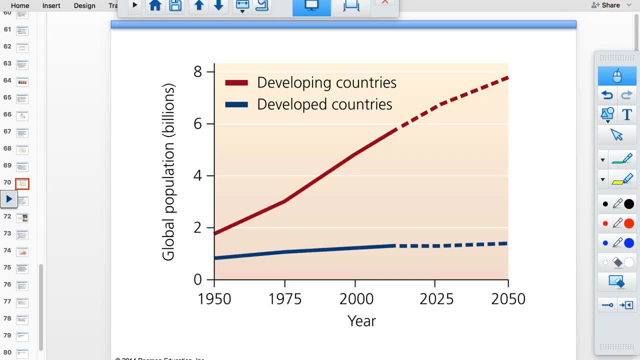 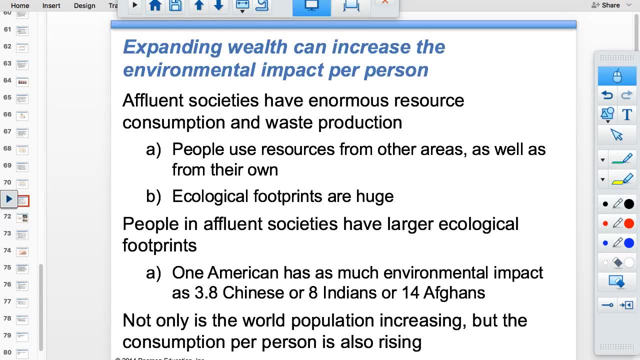 Developing countries. Again, their growth rate is a lot. Developed countries not grown. 99% of the next billion people will be added to countries that cannot support them. So affluent societies have enormous resource consumption. One American has the ecological footprint of eight Indians. So we can sit here and be like 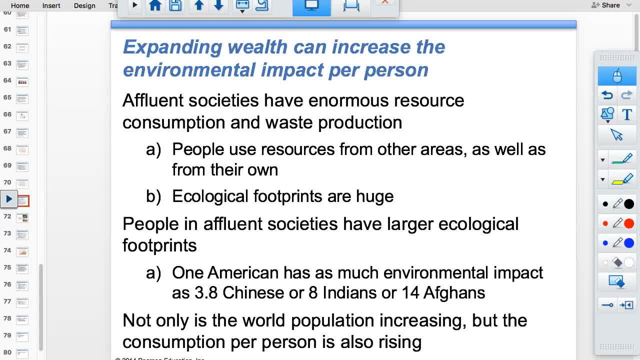 well, if you do the math eight times 300 million is 2.4 billion. What's the population in India? 1.2 billion. So is our footprint larger than India, even though they have 200 million people? Yeah, by a lot, By twice as much, even though we don't have as many. 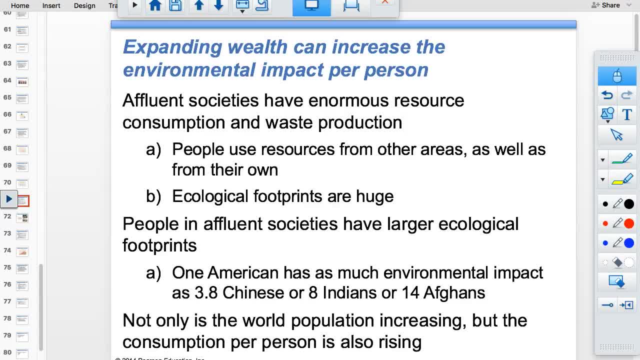 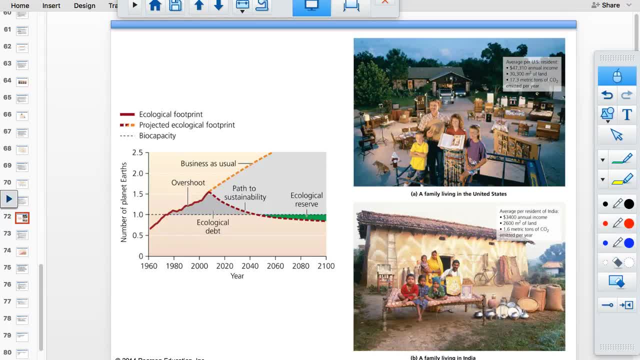 people. So population in and of itself is not the whole, the whole issue. So all right, here you can see that graphically- a family in the United States. I hope they have money to help them take everything they own outside Here. the neighbors will come and go and we'll go to the grocery store. How much for a couch? 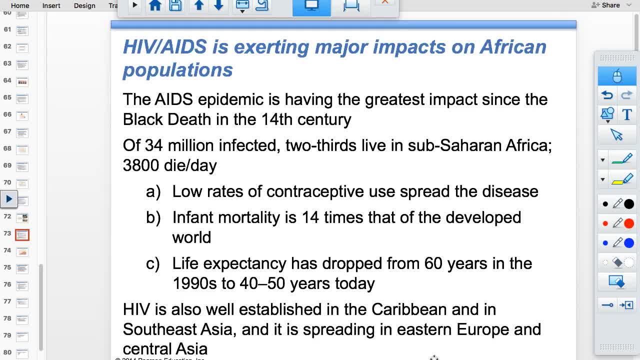 And there's the average Indian family and what they have, I don't know. Age is kind of perplexing and that means obviously you know tragic and you know not good things, but the AIDS epidemic is having quite an impact on population and so when I showed you the demographic transition, the first thing that drops is: 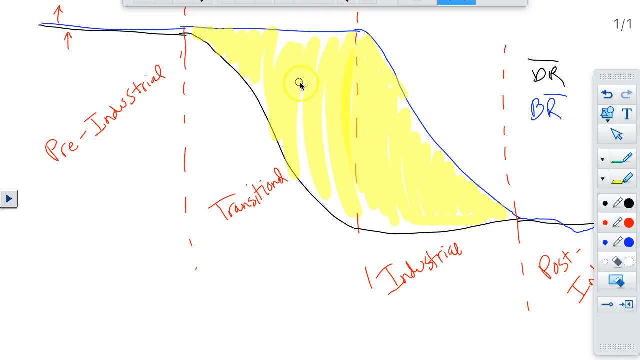 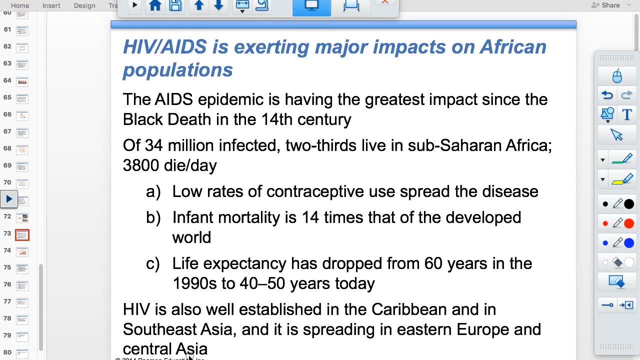 death rate. well, guess what if your country has an AIDS epidemic going on? in some areas, one in three people have AIDS or HIV. one in three, okay. so that is killing a large portion of people. and in some developing countries, especially sub-saharan Africa, the the life expectancy is in the upper 30s, low 40s. 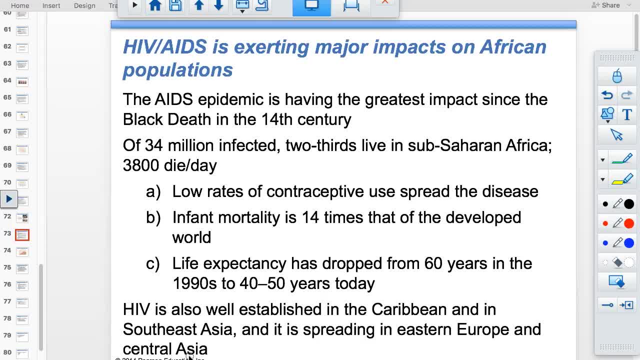 now like, instead of being like, the United States in the 70s, low 80s. in some countries it's in the 30s and 40s because of AIDS. and so if we have to drop the death rate before, you can drop the birth rate, but you can't drop the death rate because you have AIDS. 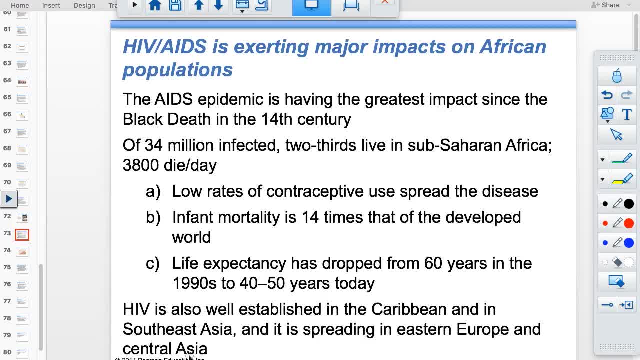 right and so these problems just keep getting exacerbated. the reason this is an issue- low rates of contraceptive abuse because of patriarchy, society, but then also infant mortality rate is as higher again, can't get that drop, that birth rate to drop and so the life expectancy. and, like I said, in some countries, in some areas, 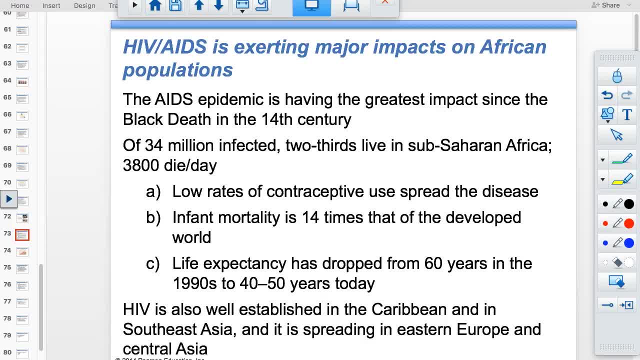 it's less important for life expectancy now and this goes back to some kind of cultural myths in some areas. I have a friend that she worked for the CDC and she did some work. she actually got malaria when she was in Malawi. this works with start with the 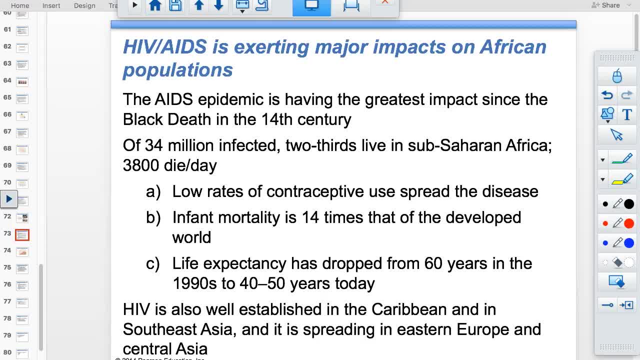 male, but whatever she was telling me that they have, and I think it's in the half the Scottie, there's this cultural belief that if you have sex with a virgin you can't have AIDS. and so you. this is rampant rape of children, even really, really young children, and this 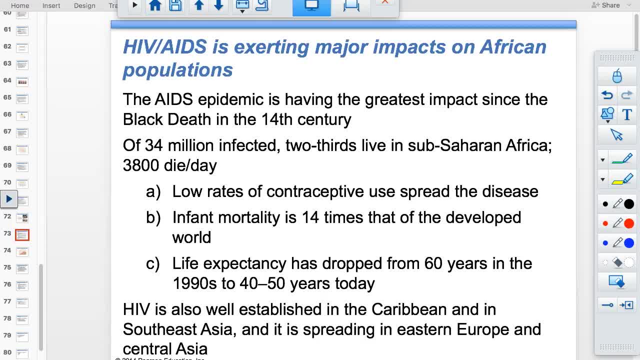 that obviously doesn't work. and so then you have, and AIDS infected children. well, and these countries, they can't afford the medicine for the people and the people in a country. if you think about it, this is the impact: the people in the country that are really the tax base, that are that are working. 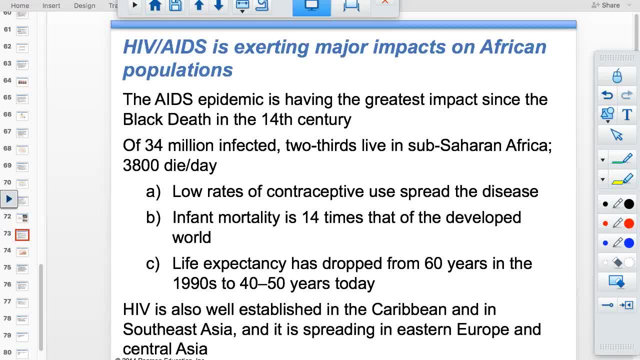 to contribute to the economy are the people that are of sexual activity right age, like sexually active age. so those people, the ones that have AIDS, and so they're dead or they're dying or they're sick or a lot of them are, and so you can't grow your economy and take care of the children and take care of the sick. 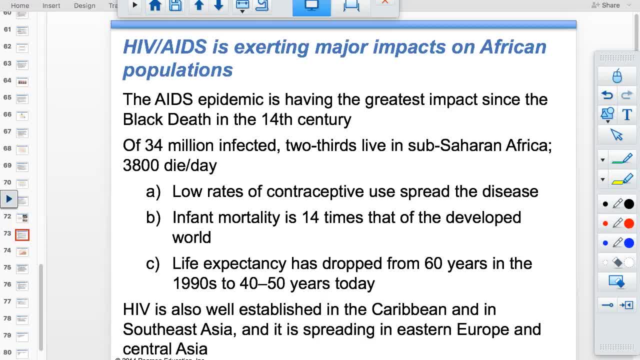 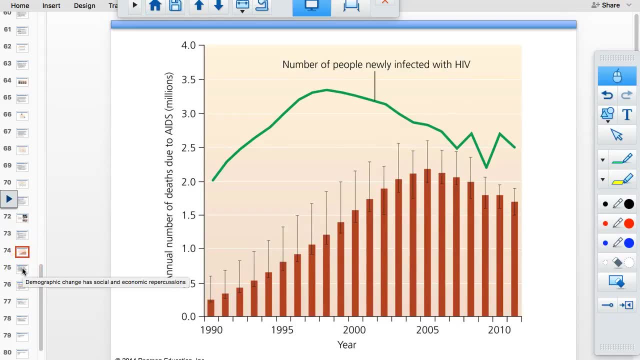 because the people that should be providing for your tax base are sick, see? so that's called demographic fatigue, which I feel like is on the next slide or two. I have a tendency to do that. let me explain everything before I get to it. so the number of people HIV is actually going, newly infected people's going down. 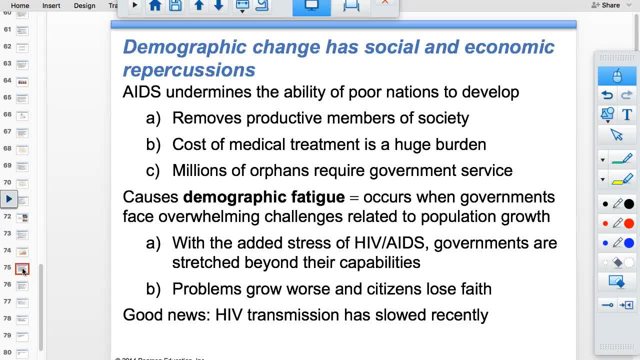 but yeah, demographic fatigue is when governments face overwhelming challenges related to population growth and so, like I said, that is the issue there, because the cost of medical treatment is huge. first, demographic fatigue is also relevant to China, because they have such an aging population and they have to cut. 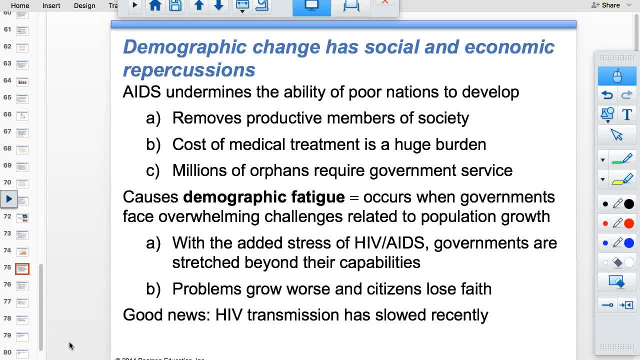 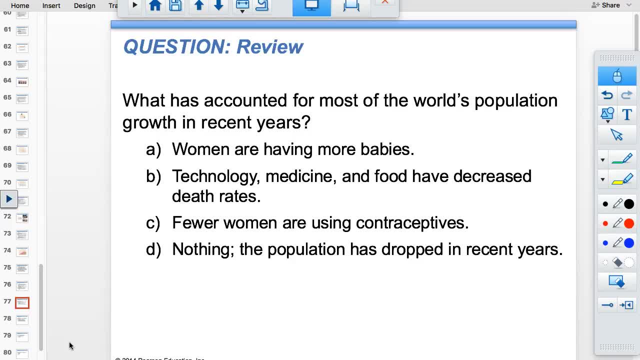 their birth rate so much so- that's another example- doesn't have to be AIDS related. so let's go over these last couple questions. what has accounted for the world most of the world's population growth in recent years? what you got Jordan, yeah, technology, medicine and food, and so the death rate- right that's. 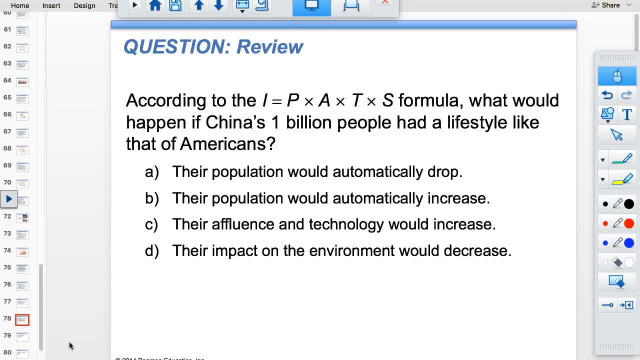 internationally kind of where we are. death rates are down. birth rates are still up in some areas, according to the IPATS formula. what would happen if China's 1 billion people have the lifestyle of that of Americans? we should. that's all correct, Lauren, what you got, well, the population affluence actually lowest. 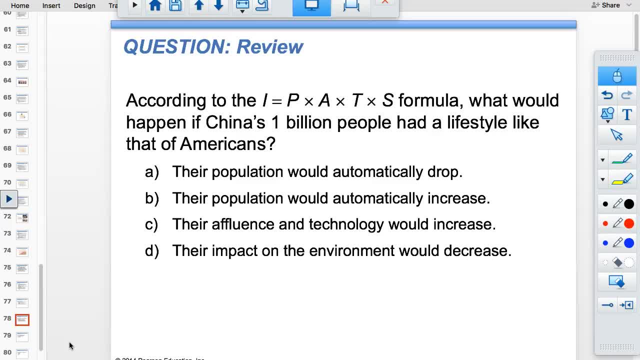 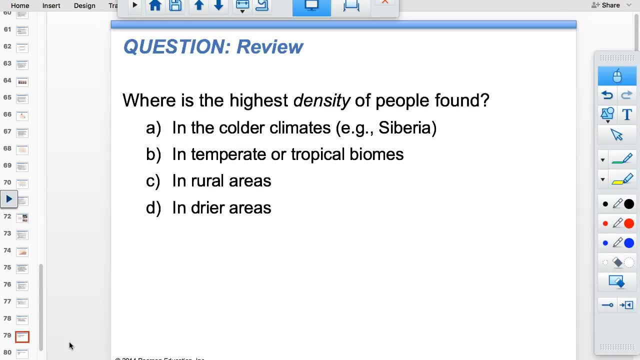 population. so maybe is there a better choice. yeah, yeah, so their affluence in technology would increase. sure, what? where is the highest density of people found? probably not Siberia. so yeah, oh, look at this, you got these so intemperate or tropical bomb shotre and a structure diagram shaped like a 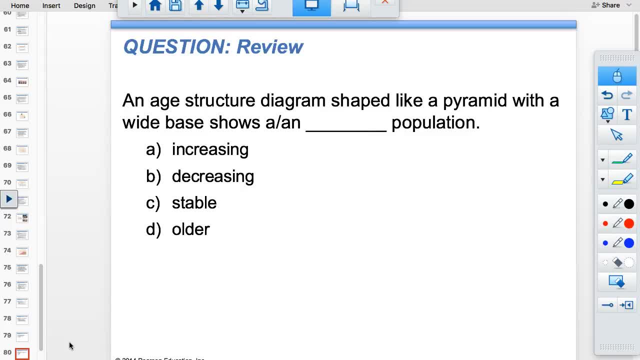 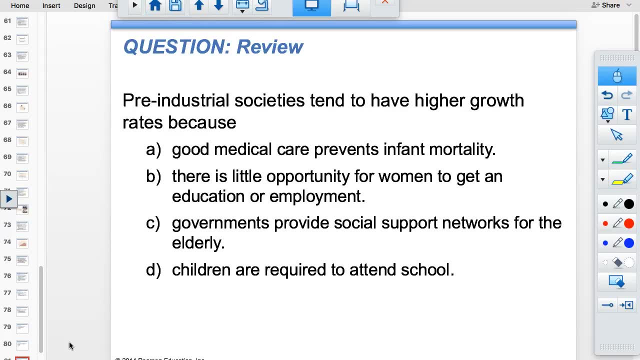 pyramid in the pyramid and it shows what happened with the population. Erica, what you got? yeah, sure, pre-industrial societies tend to have higher growth rates. b because it increase again. yeah, children, all the B. today, when children of tiene are the vasel changed to a better waste culture next year, for example. 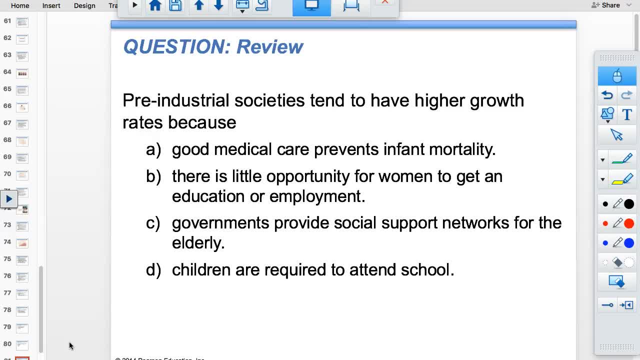 trying to include generated very passive collection to be the ideal thing to you know you can worry about. what have you given me? B, two years a full jump juga, yeah, actually, or wait. B is why I'm missing these consulting name for really in one of my kids. you know who. 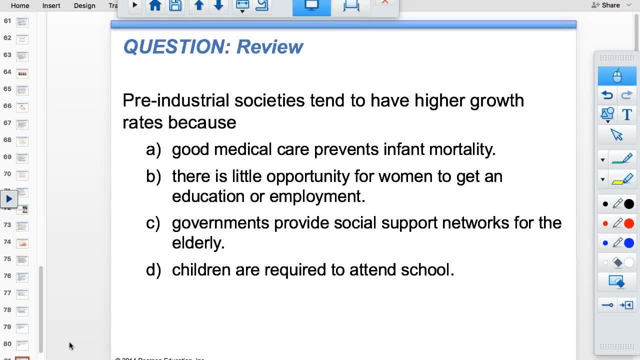 But first and foremost, everyone has become囧- your case children, almost just over 50-60 Consumer. wait, which one B? You said B like boy, right, Okay, good, There is little opportunity for women to get an education or employment. 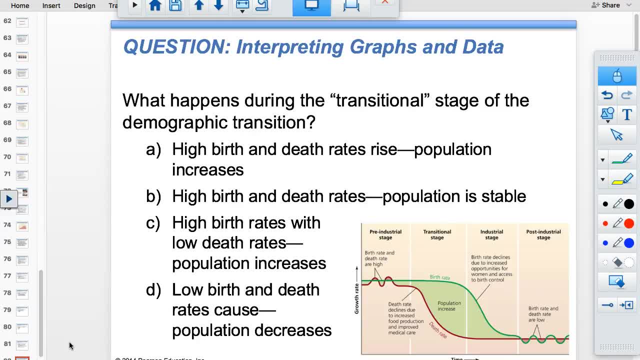 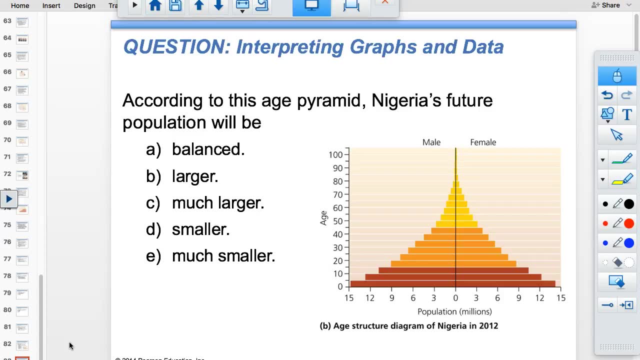 So what happens during the transitional stage? the demographic transition? What say you, Skyla? Yeah, so high birth rates with low death rates, and the population is going to increase, So we should all feel pretty good about that. According to this age pyramid, Nigeria's future population will be: 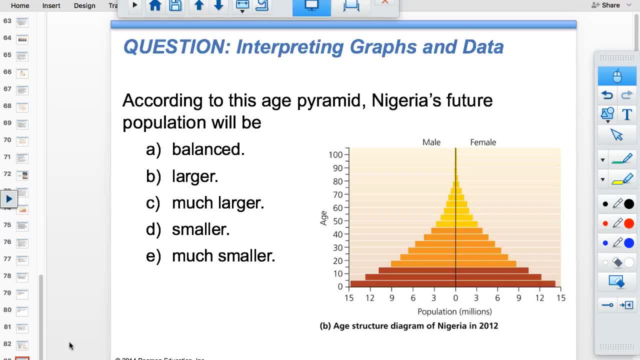 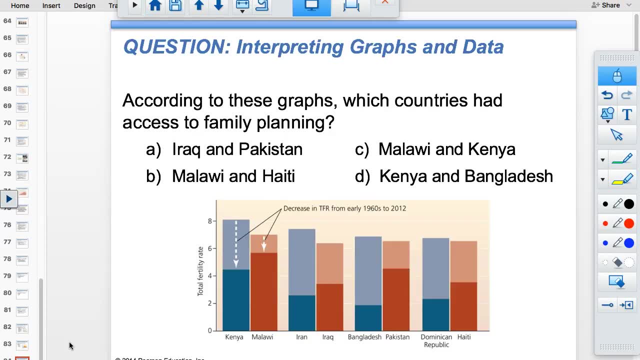 keeping the same person that's out here. It's pretty funny, Ezra, what you got. Yeah, much larger, Larger, much larger. And so, according to these graphs, which countries had access to family planning? I'll give you a second to look at this. I don't know if you got to it earlier.